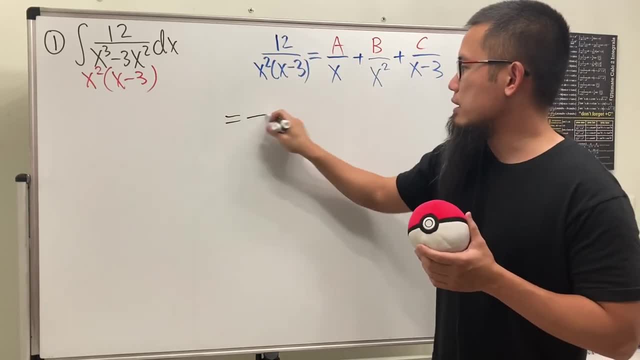 as. if you don't want to build up the power, then just put this down as x squared here, And then plus this right, here is x minus 3.. Again, we are not building up the power, right, if you don't want. 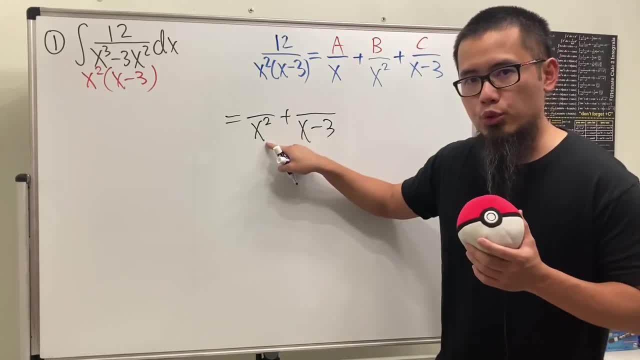 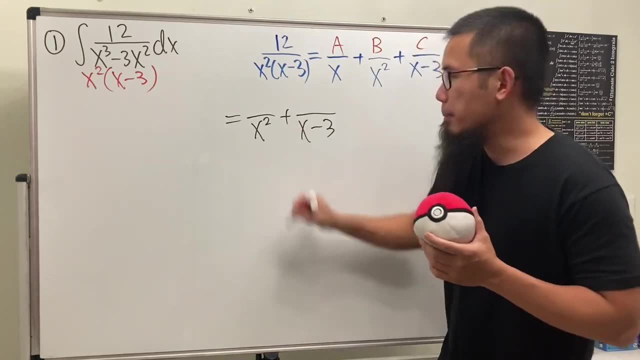 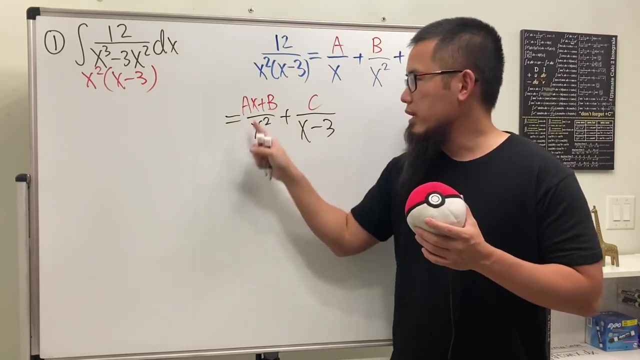 to. But if you don't want to do that, this right here, you have to look at it as a quadratic. That means the top should be a linear. So you will have to put down ax plus b. So let me just write that down. And of course this is going to be a constant. But you see, this guy, we can split. 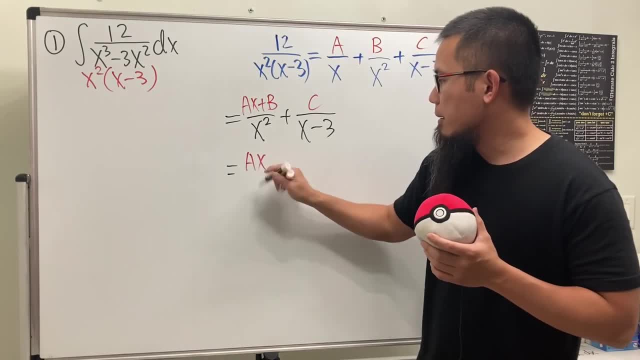 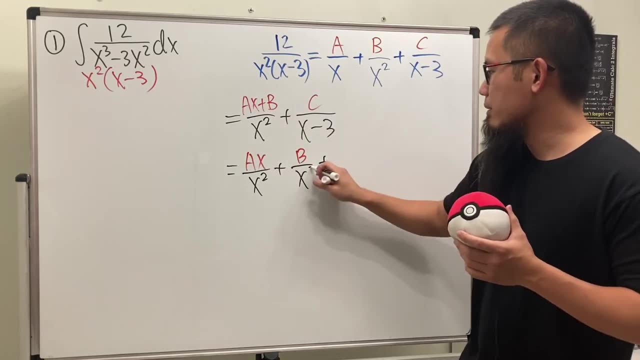 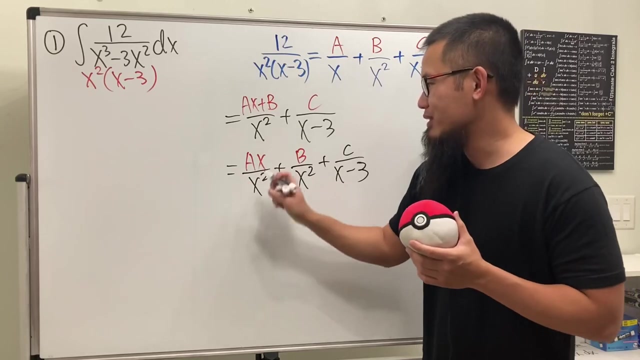 the fraction. So we are looking at ax over x squared, and then plus b over that, And of course we still have this guy c over x minus 3.. But what can we do for the first fraction? Well, as you can see, this and that cancel, And 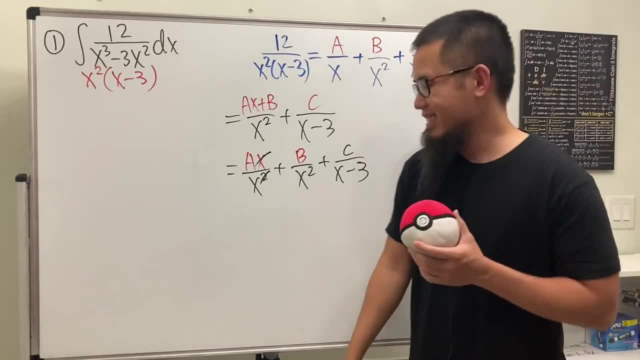 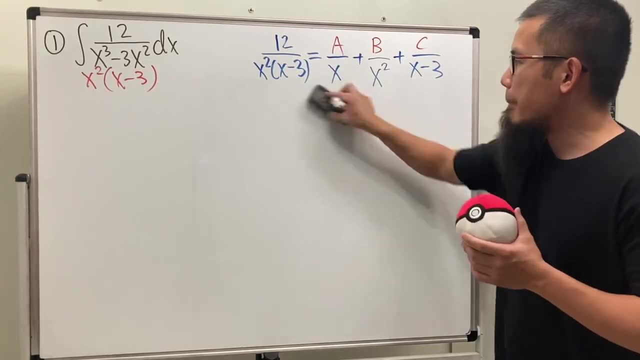 that's exactly why we need the a over x. all right, So anyway, just go from here to here, That will be it. You don't have to do this every single time. Build up the power and the top stay the same kind, And then we have this guy: c over x minus 3.. And, of course, we still have this guy. 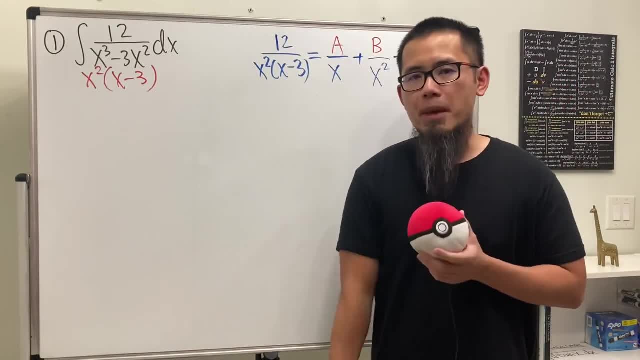 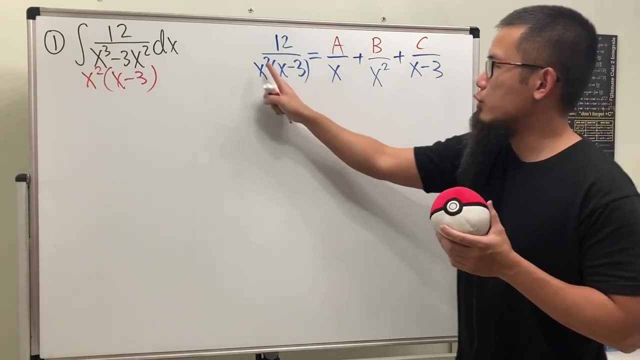 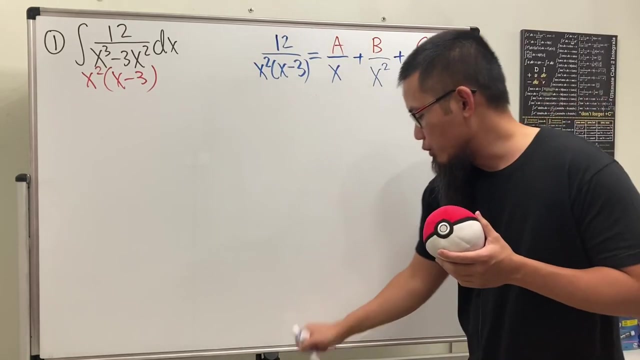 c over x minus 3.. And now, good news for you guys: We can actually use the Capra method for two letters, b and c, because we see this denominator right here And likewise we see this denominator right here. So b and c, we can use the Capra method for that. So let's go ahead and do them. 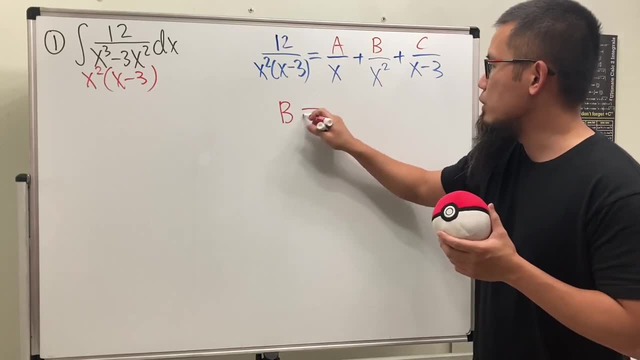 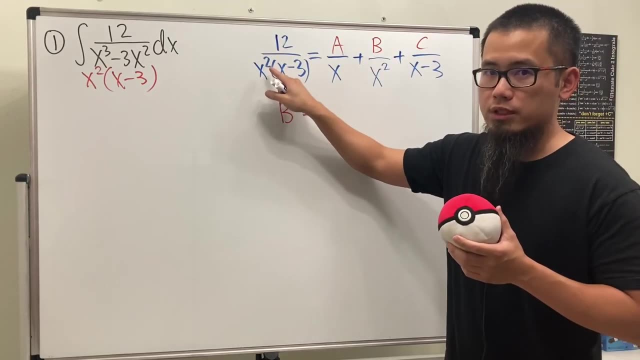 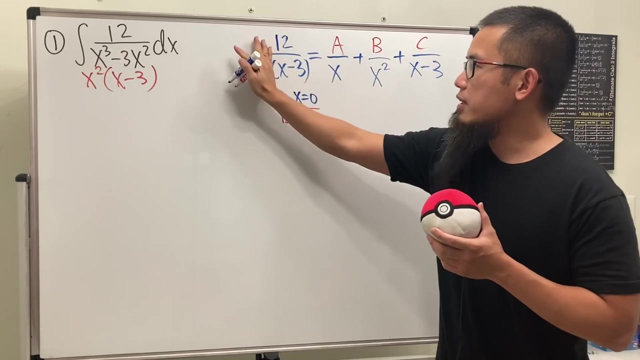 first. So let's do b. Well, b is going to be equal to. we go back to the original and we cover the same denominator. And how can we make x squared equal zero To be zero, right? So I'll just put down: x is equal to zero And we cover this up already, So we put. 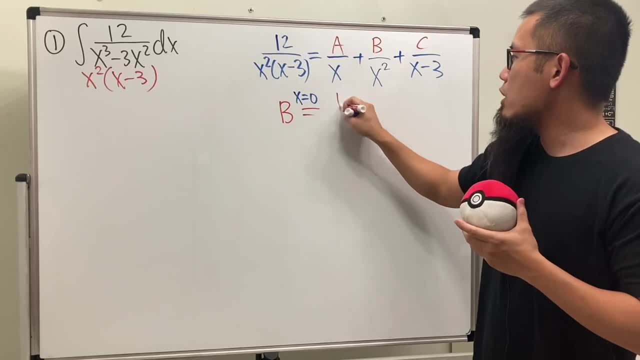 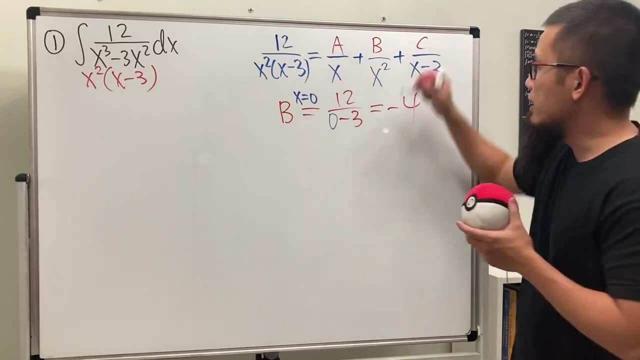 the zero into this x only, And we are looking at 12 over zero minus 3. And that will give us negative 4.. So b is equal to negative 4. And I think that's pretty good. Now for c. this is going. 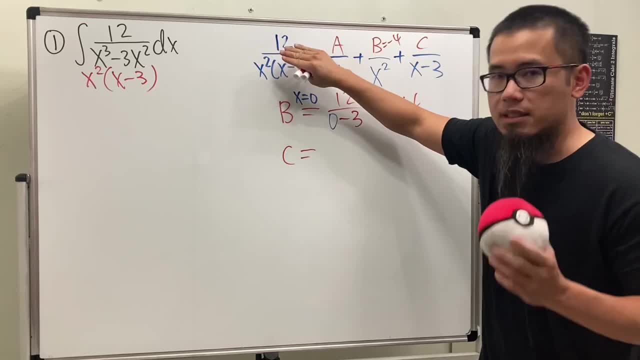 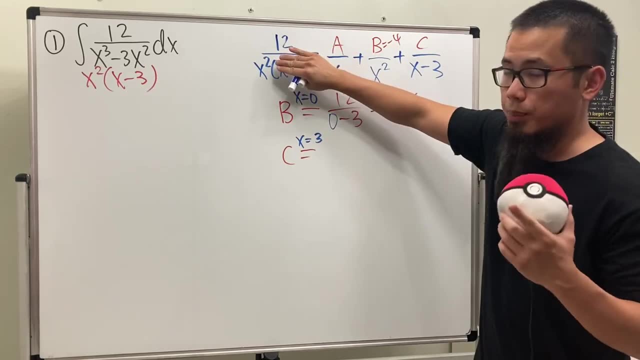 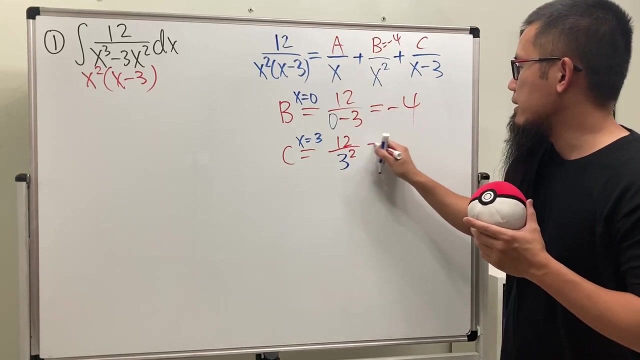 to be. we'll come here cover this up when x is equal to positive 3.. So let me just put that down real quick And we cover this up already. So we put 3 right there. So we are looking at 12 over 3 squared And 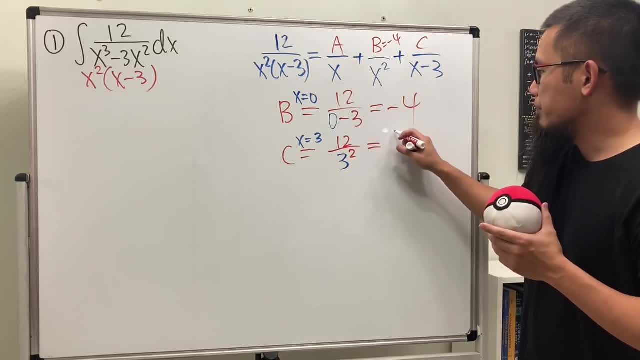 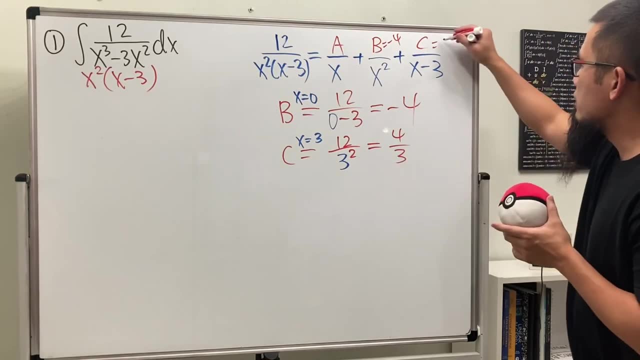 this right here is going to give us 12 over 9.. And that will give us 4 over 3 after we reduce. So we have the b and c value, which is pretty good. So this is 4 over 3.. Okay, not so bad. Not so bad. 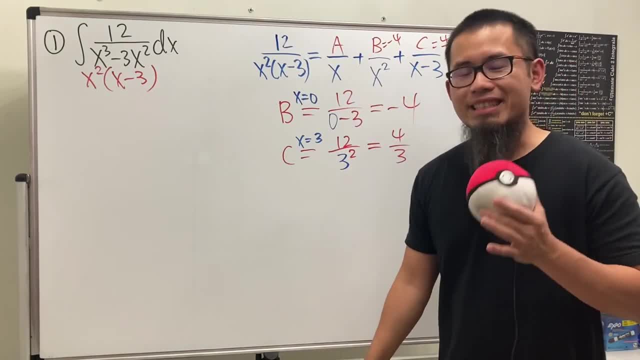 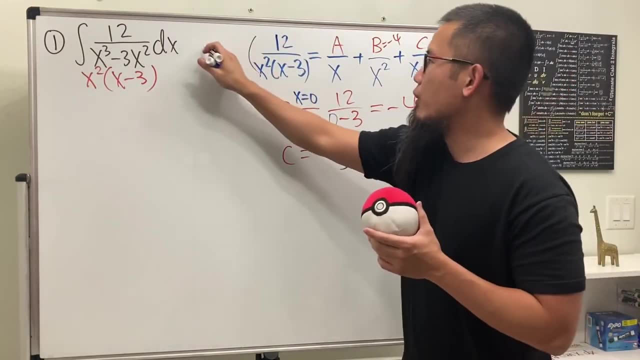 Now let's see how we can figure out the good, old-fashioned way. Let's go ahead and look at this and multiply everybody by the lowest common denominator, which is just this guy. So x squared times x minus 3.. And we are looking at this times that. 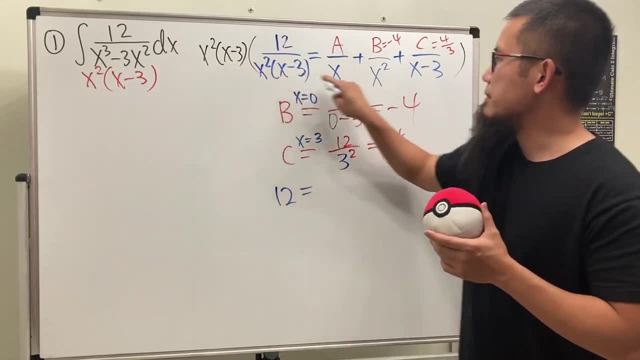 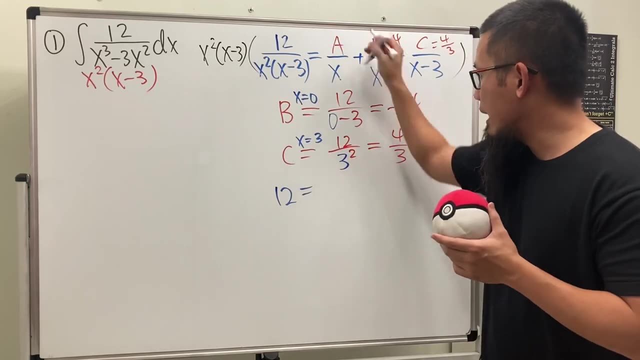 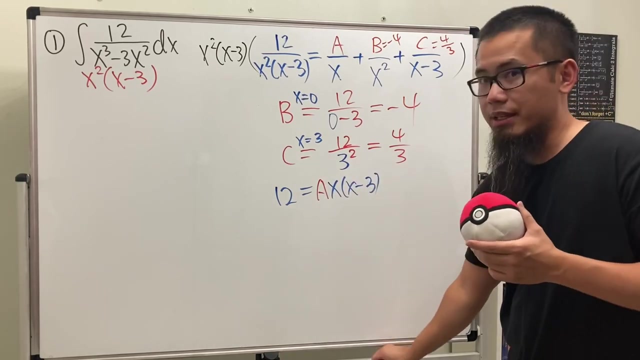 we just have 12.. And this times that, well, one of the x can. So we have x times that. So we will have a, which we don't know yet, x to the first power times, x minus 3.. And let me just 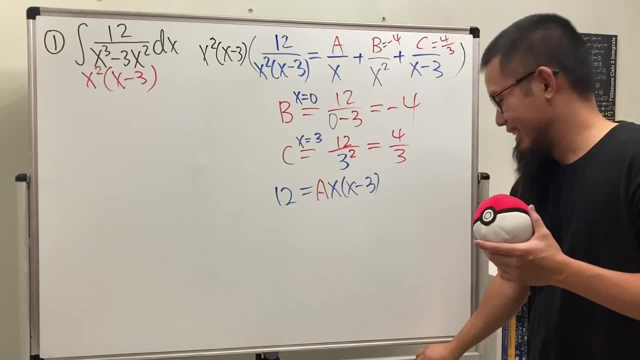 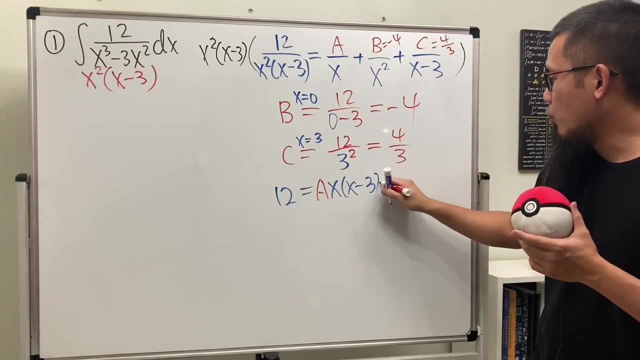 fix my exponent 2 right here real quick, Okay, Okay, next we do this times that The x squared cancel. So we will just have the b, which is negative 4 times that, which is x minus 3.. And 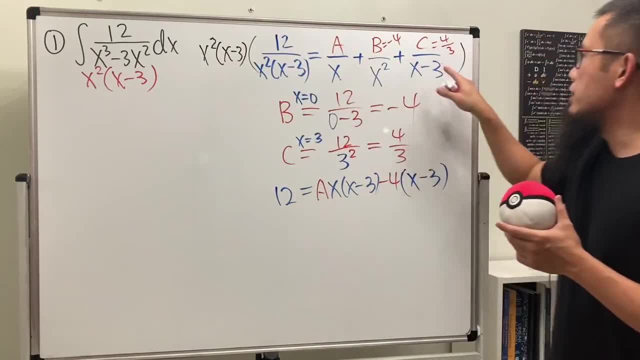 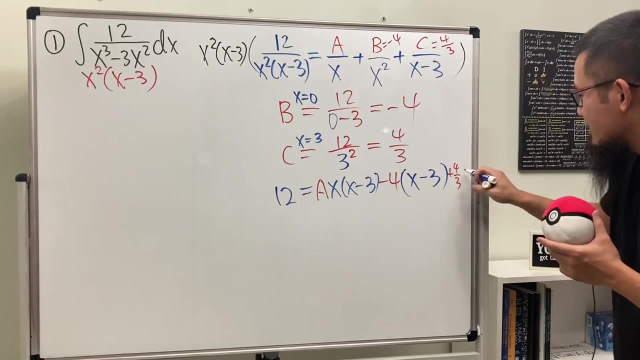 lastly, this times that the x minus 3 cancel. So we just have this, which is 4 over 3 times x, squared right here. Oh, it fits everything. So that's nice. All right, Now again, just like what we were doing in the previous video. 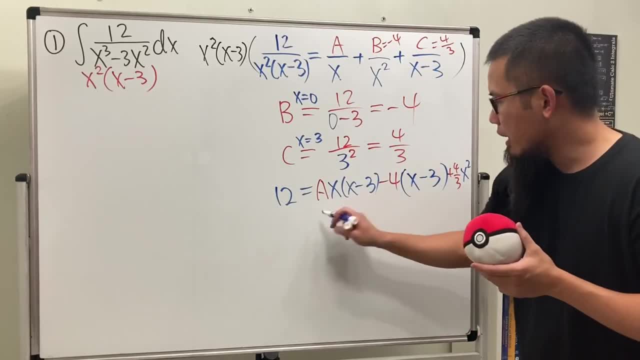 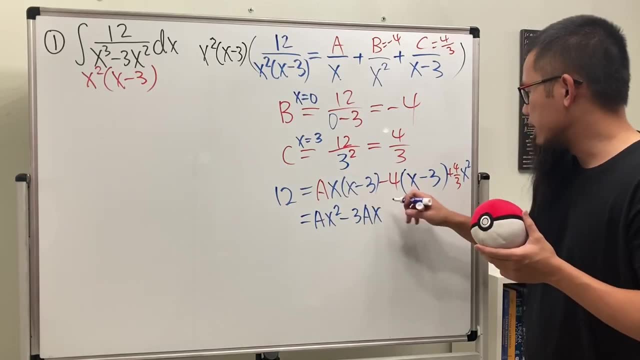 just go ahead and multiply this out and try to look for what a is Okay Here. this is going to be a x squared and a minus 3 a x, And then, in fact, you don't really need to do anything but. 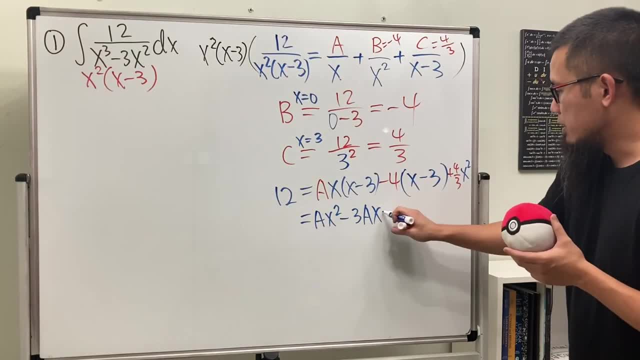 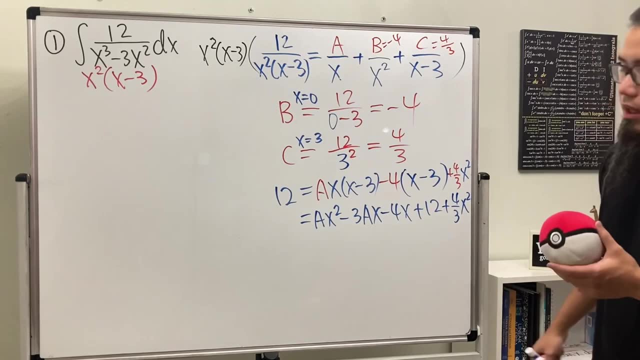 like, let me just finish this real quick. Let me just finish this. This is minus 4x, plus 12.. And lastly, we have the plus 4 over 3 x squared, The reason that I said we didn't really need to do. 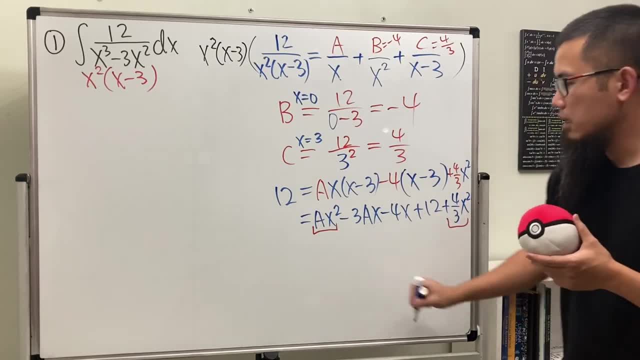 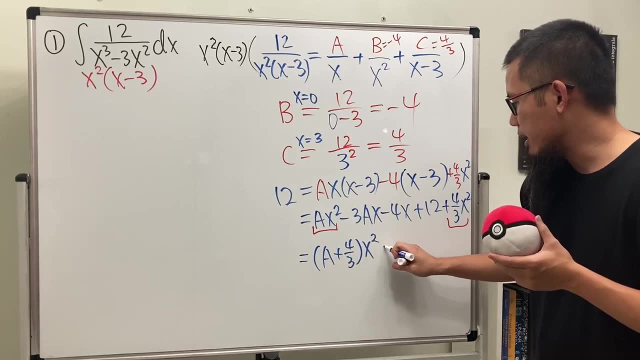 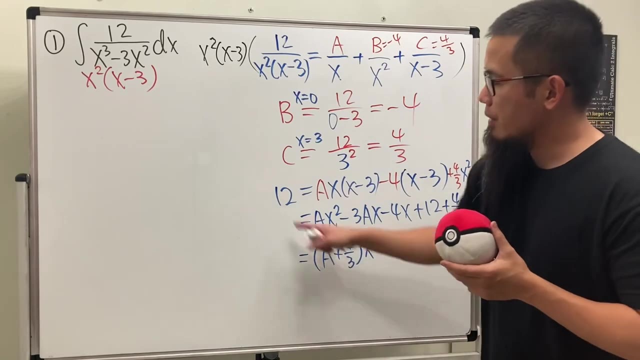 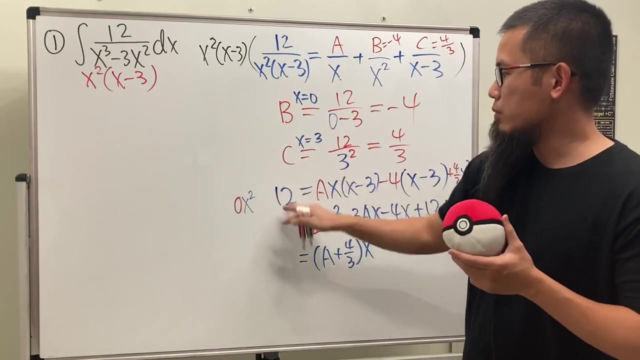 is because we can just look at this and that This right here will give us a plus 4 over 3 times x squared, and then other stuff. We really don't need any of them anymore because this right here tells us because on the left-hand side we pretty much have 0 x squared right, Because there was no x. 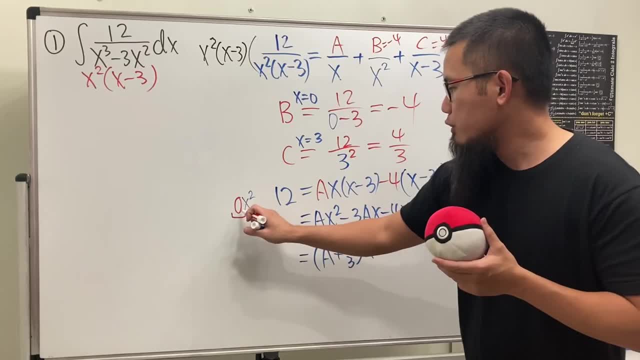 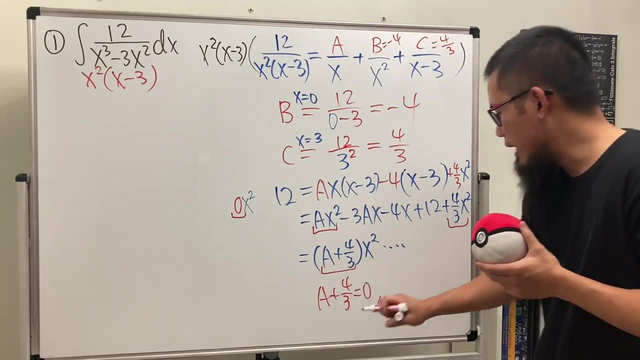 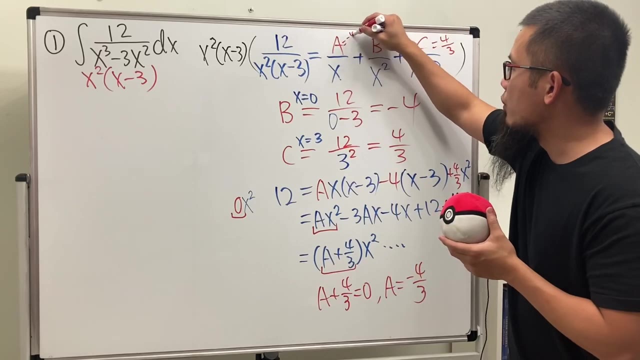 squared term in the first place. So that means the coefficient right here is zero. So this right here should be zero. a plus 4 over 3 is equal to zero. That means a has to be negative 4 over 3.. So we can just come here and say a is equal to negative 4 over 3.. 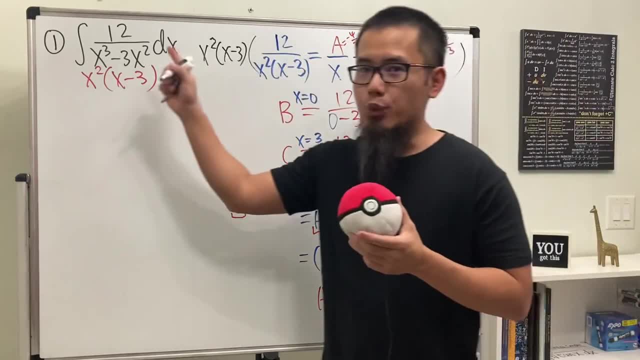 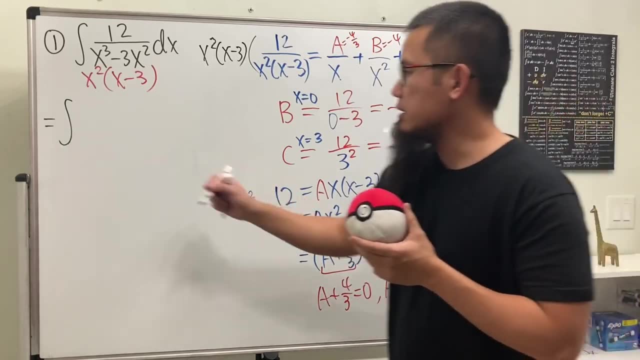 Cool. So now to integrate this guy, it's going to be the same as integrating the first guy, which is negative 4 over 3.. I'm just going to write it down like this: Negative 4 over 3 over x. 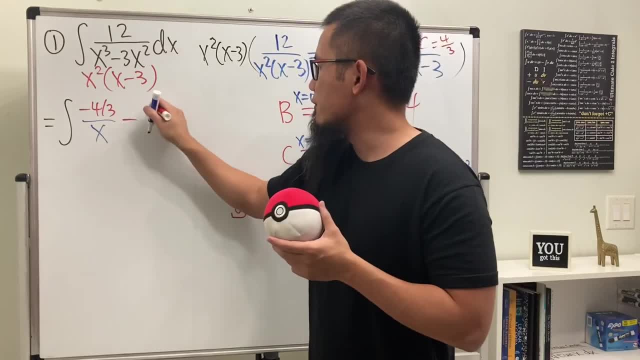 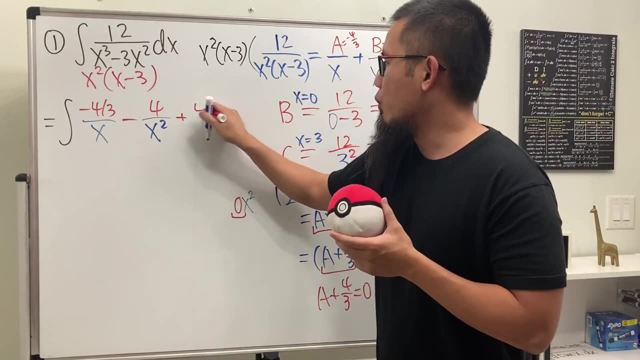 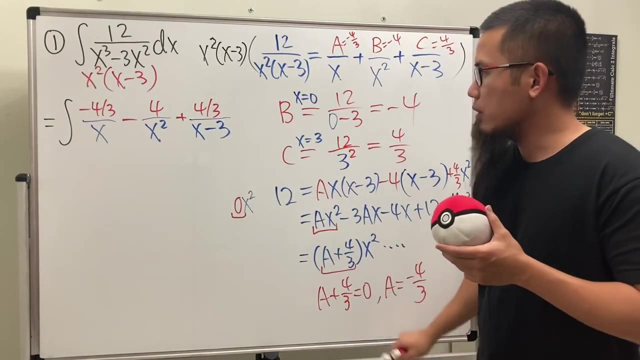 Next we have negative 4 over that, So we will have the minus 4 like this over x squared, And then that guy is going to be plus 4 over 3, over x minus 3. So that's about all, And then perhaps 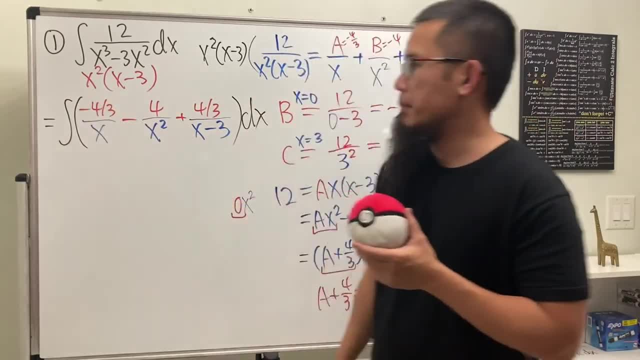 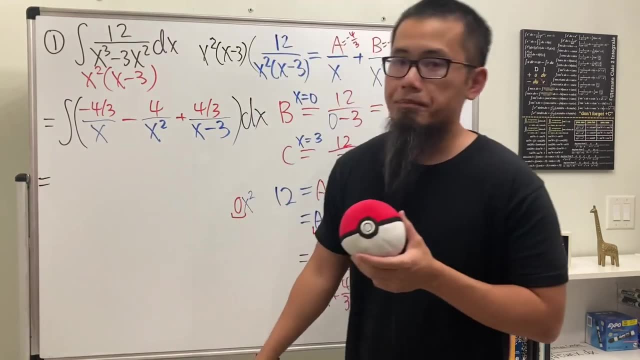 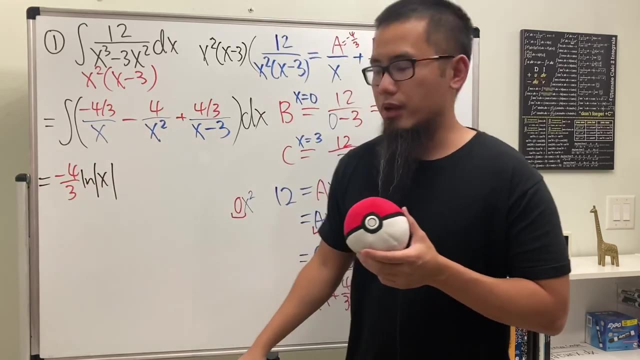 I'll put on a dx right here And, just to make more people happy, I'll put on the parentheses over there And, of course, we'll just finish everything right. Let's just go ahead and integrating everybody. First guy: Negative 4 over 3 ln. absolute value of x. Next guy: Well, let me remind you guys this real quick: 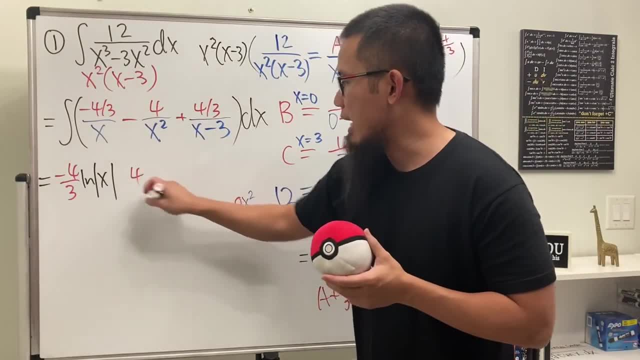 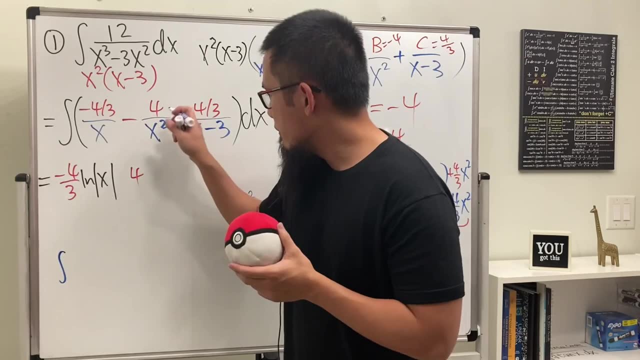 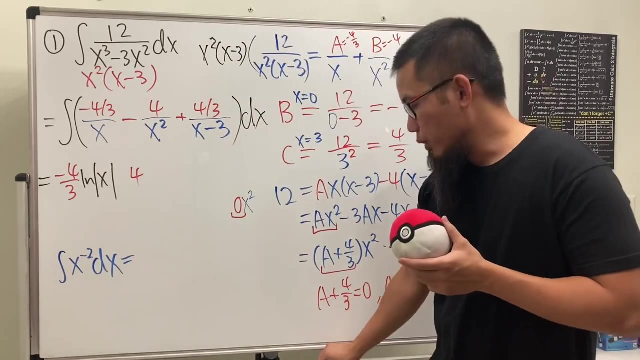 We do have a constant multiple of 4 right here, so we can put that down. But I will remind you guys: the integral of the 1 over x squared, which is going to be x to the negative 2.. This, right here, we do the reverse power rule. We add 1 to the power which is going to be. 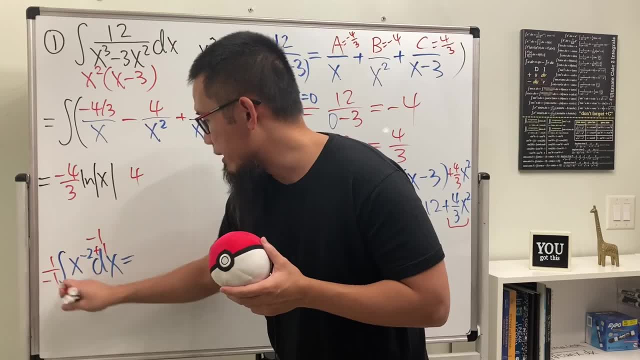 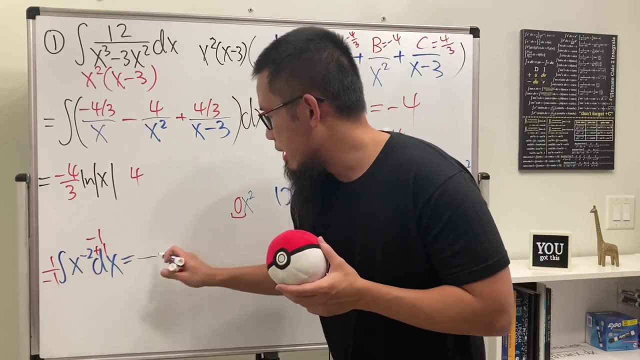 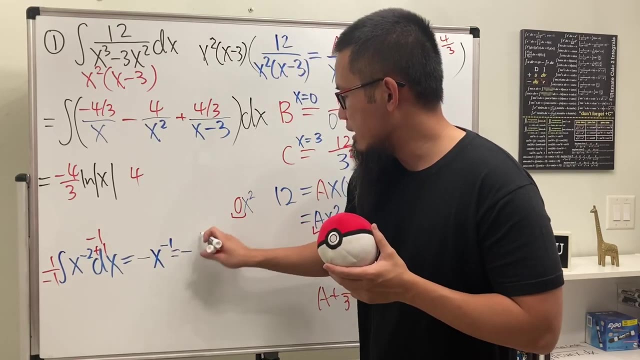 1, and divide it by this power, So we will have 1 over negative 1.. And this is going to give us negative and x to the negative 1 power. So let me just write that down And that's going to be negative 1 over x. So, as we can see this right here is negative. 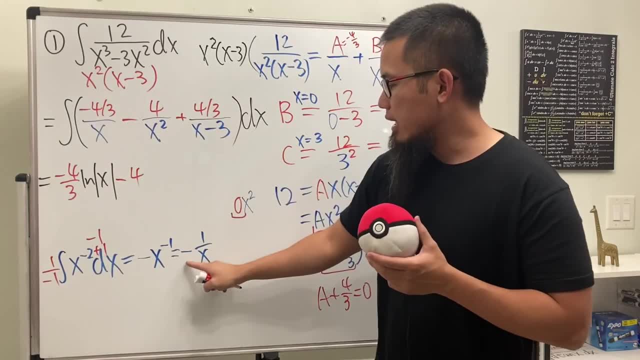 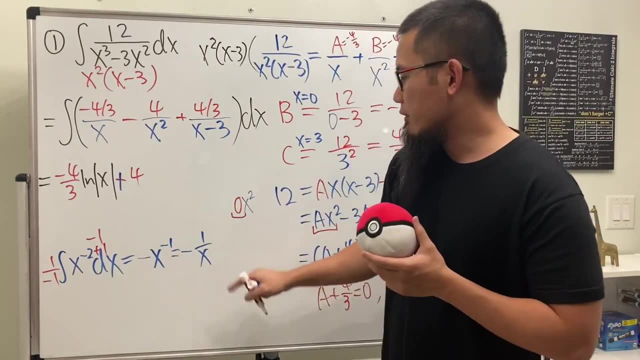 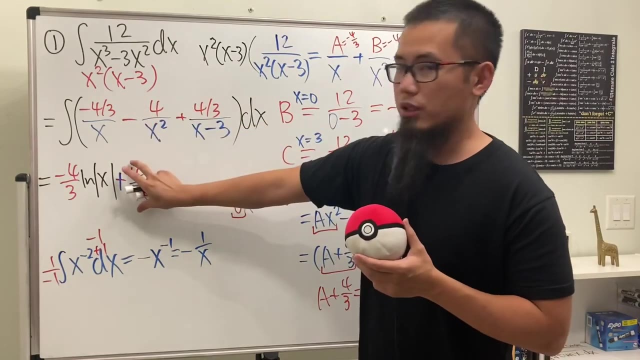 But if you look at the integral of 1 over x squared, we get negative. 1 over x. Negative times 1 over x squared gives us positive right there, And then, of course, we can also put down the over x like this: So this integral is going to give us that, And then, lastly, we'll 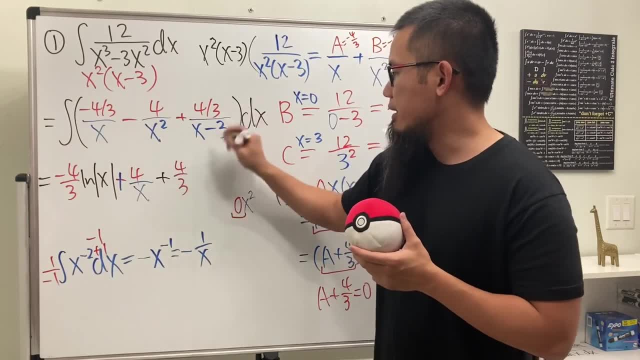 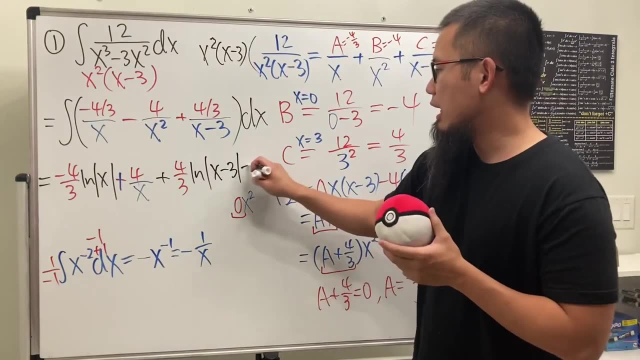 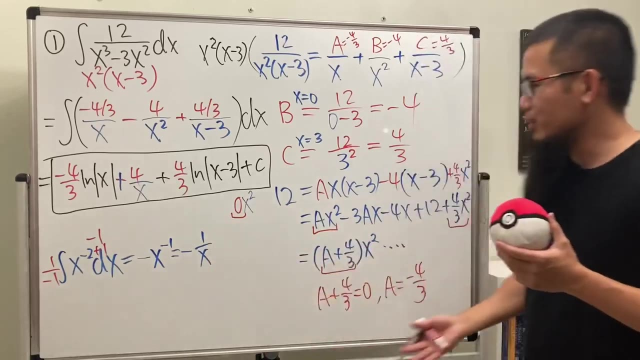 just add 4 over 3.. And then again the bottom is just linear. So ln absolute value of x minus 3.. We are all done After we put down the plus c. this is it, So take a look right now. 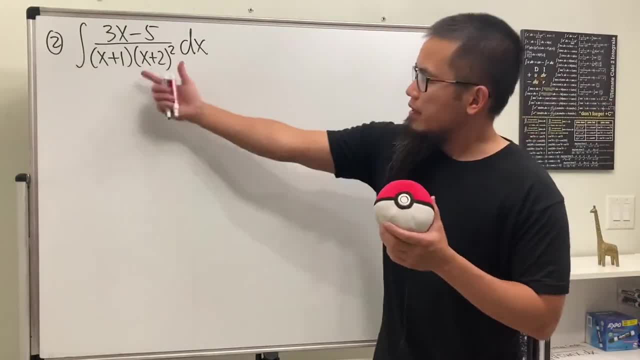 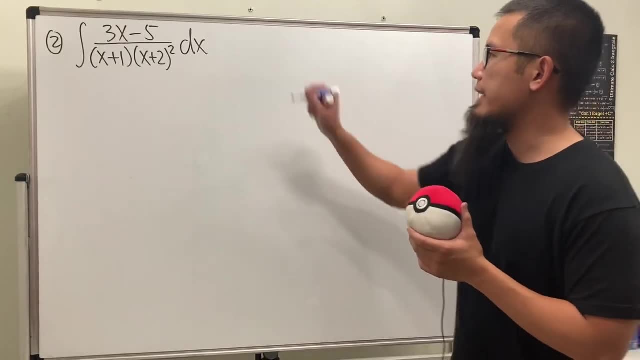 Right here real quick. Okay, question number two: The denominator has been factored in for us already, which is very nice, So we can just go ahead and do the partial fraction, And of course that's doing on the side. 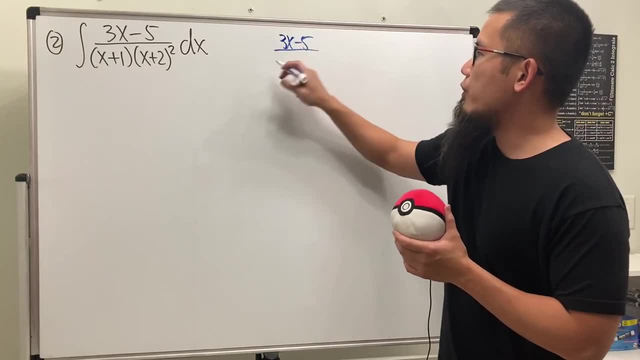 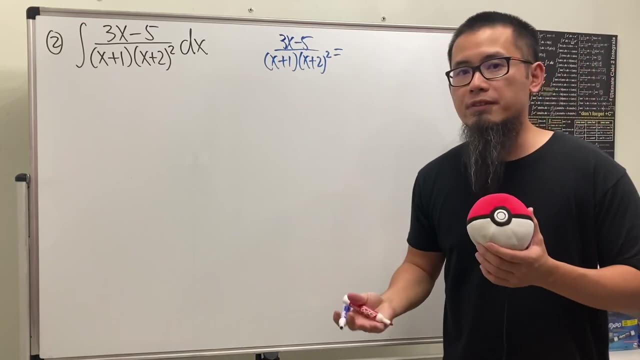 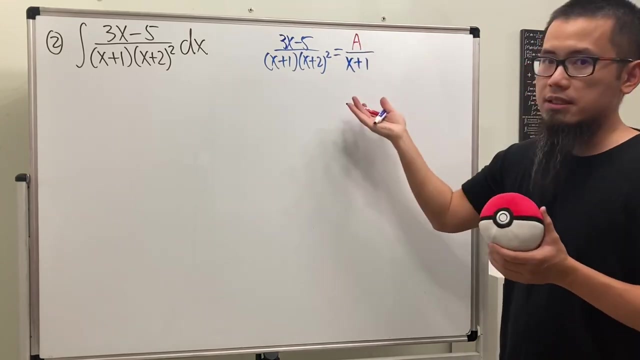 We are looking at 3x minus 5 over x plus 1 times x plus 2 squared. So right here this is the repeated factor, right. First we will have this for the denominator And that's just x plus 1.. And the top will be just a constant. And for this part, 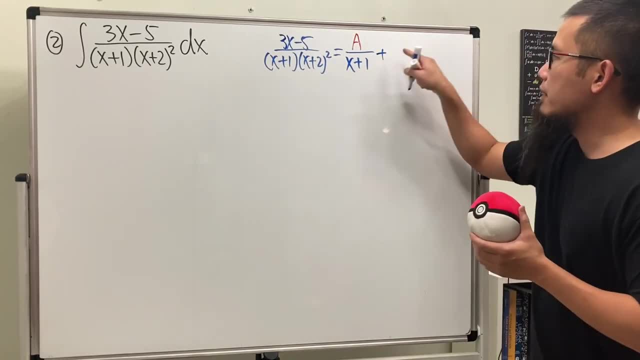 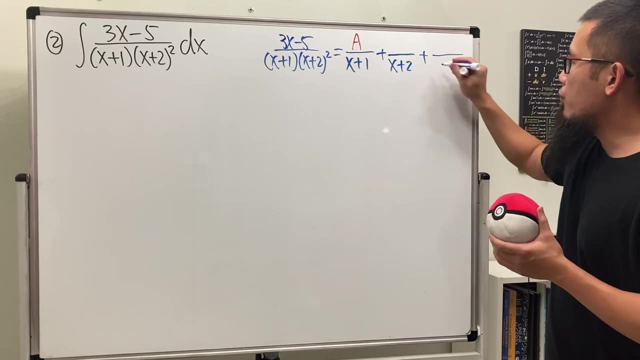 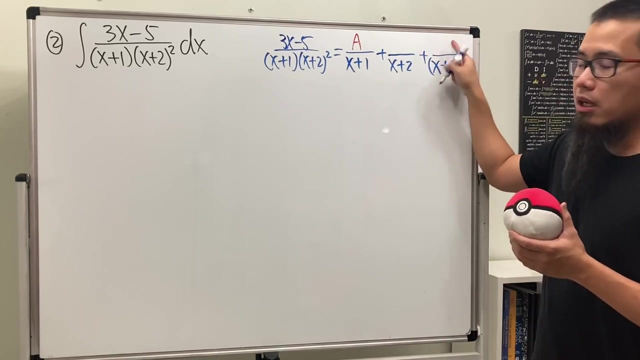 we will have to build up the power. So we are going to have some number over this, which is x plus 2.. And then some other number over x plus 2, squared right. We put down the power And I said this is the number, And this is the number because, well, this is linear, That's. 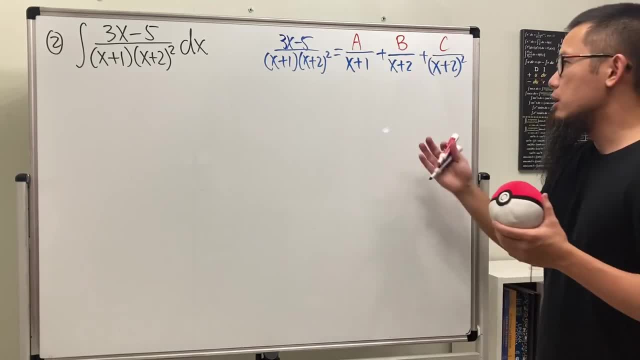 why? And then the top stays the same kind. So let's put down b and c, So that is what we have. And now let's multiply everybody by the. Well, actually, no, not yet. Let's get the. 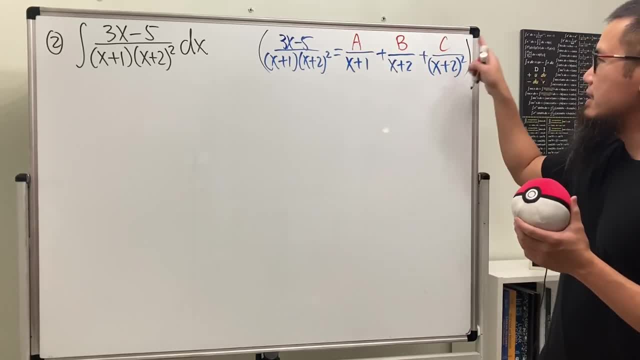 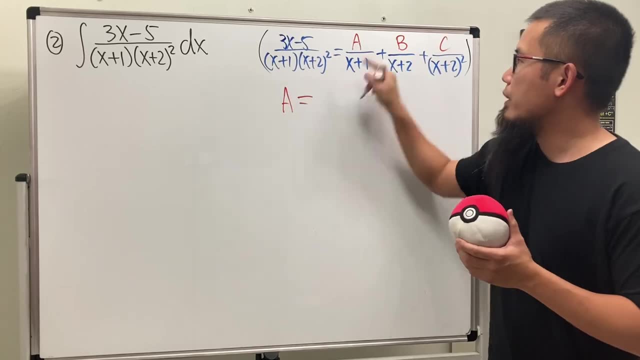 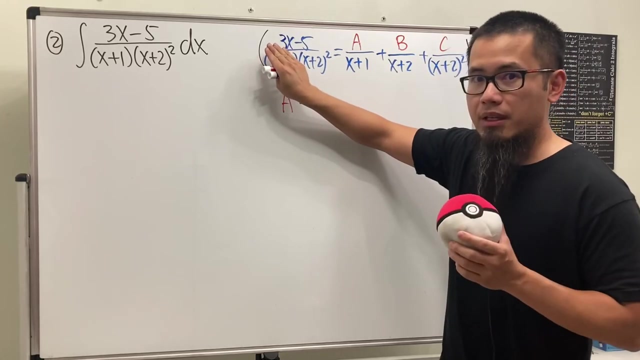 Let's get a and c by using the cover-up. So here we go, To get a with the cover-up. well, this is what we do. The denominator here is x plus 1.. We go back to the original cover, the same denominator. And how can we make x plus 1 equals 0? x has to be negative 1.. So we 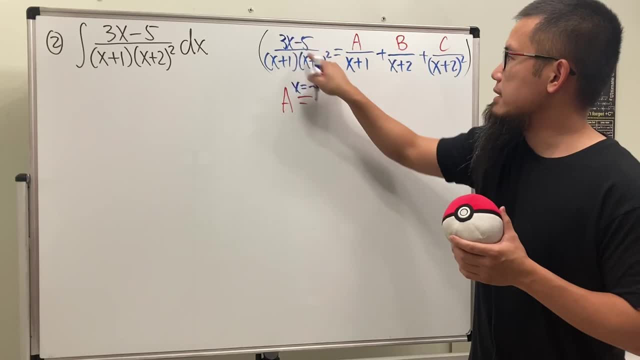 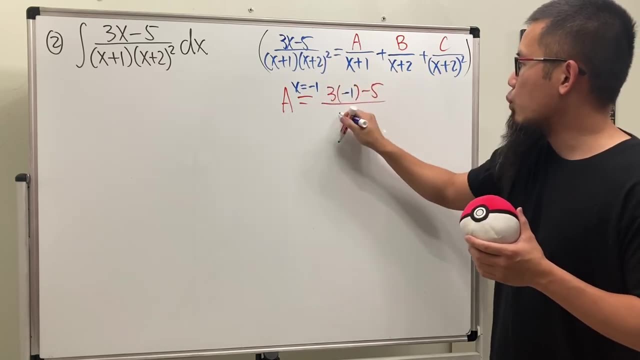 will put x equals negative 1 into this x and that x. So we get 3 times negative 1.. Minus 5 over negative 1 and then plus 2.. And then we square On the bottom. this is just one. 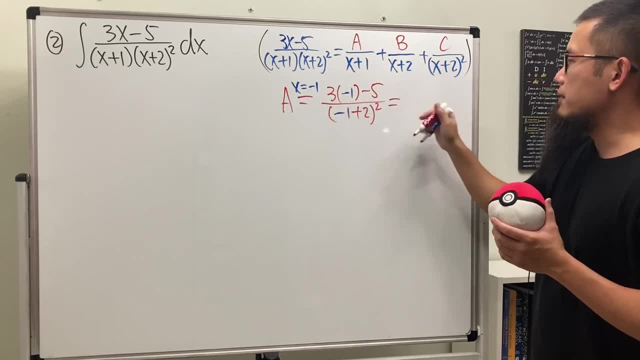 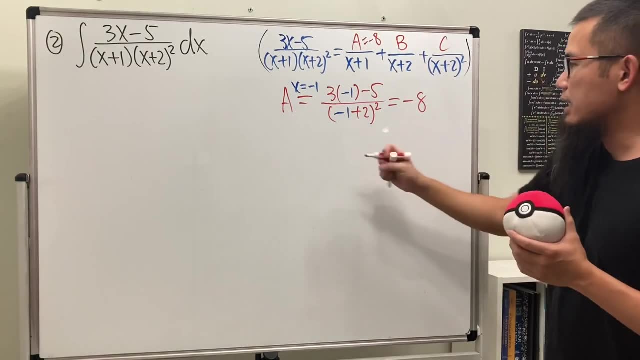 square, which is 1.. On the top, it's going to be negative 3 minus 5,, which is negative 8.. So a is equal to negative 8, which is very nice. All right, Now let's do c as well, And the reason that we can. 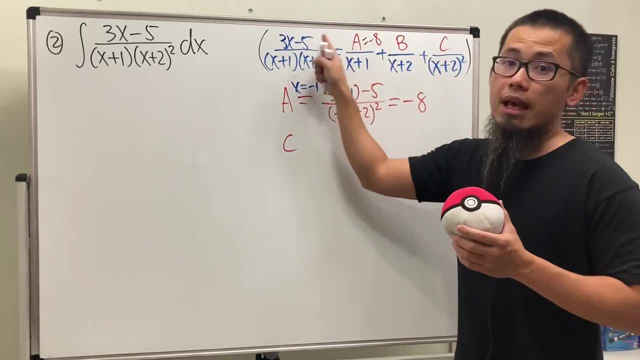 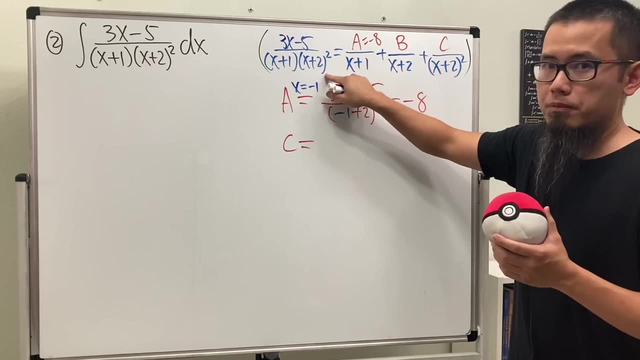 use c is because this denominator is exactly the same as this 1, right. So we cover this up And this factor equals 0. The answer is x has to be negative 2.. So we just let x equal negative 2.. 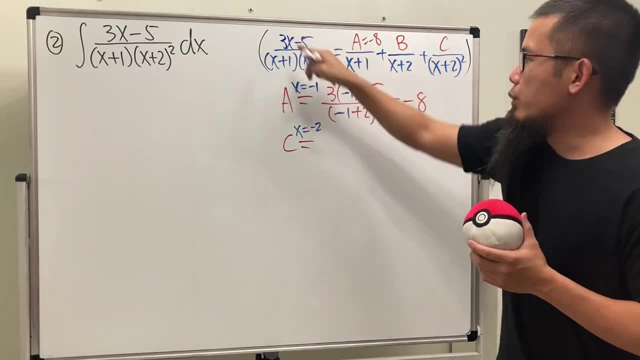 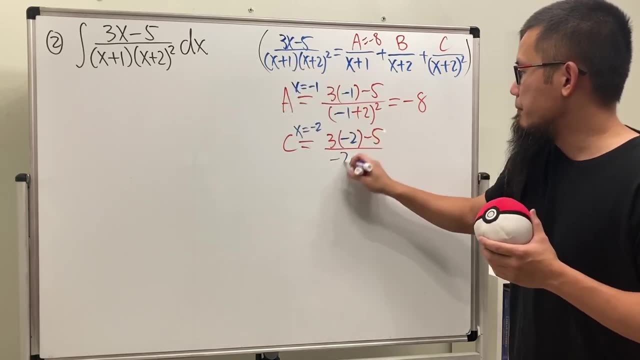 Put it here- and put it here because we covered this up already- And we get 3 times negative: 2 minus 5 over negative, 2 plus 1.. On the bottom: here we get negative 1. On the top, right here. 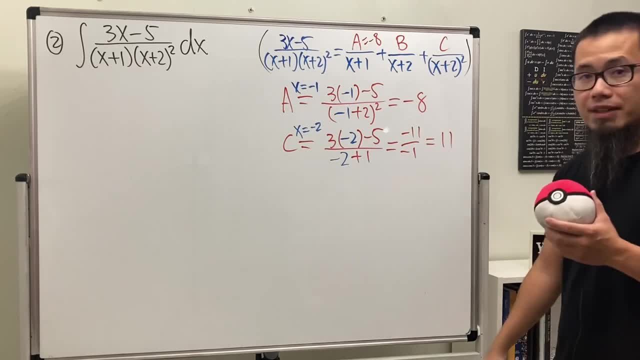 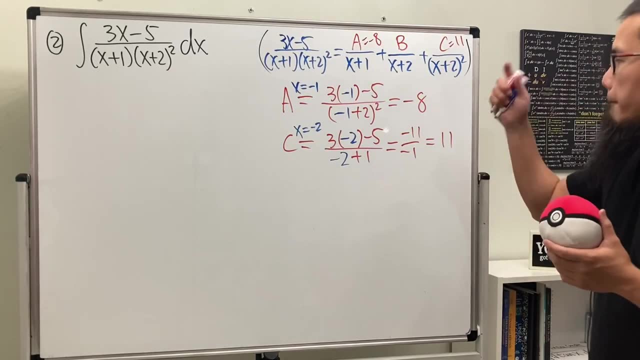 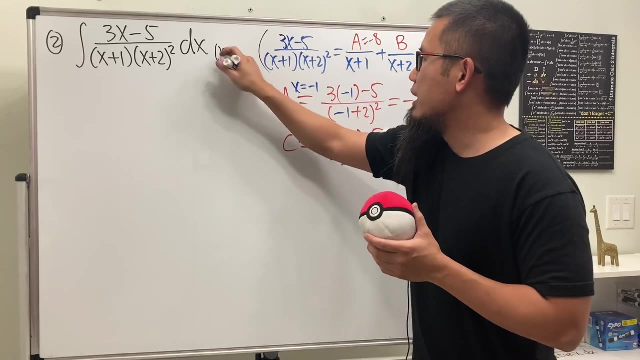 we get negative 11.. So altogether, we get positive 11.. So c is positive 11.. Okay, So that's what we have. And now to get b, let's see what we get. Okay, Multiply everybody by the common denominator, which is x plus 1, x plus 2 squared. This times that we just get. 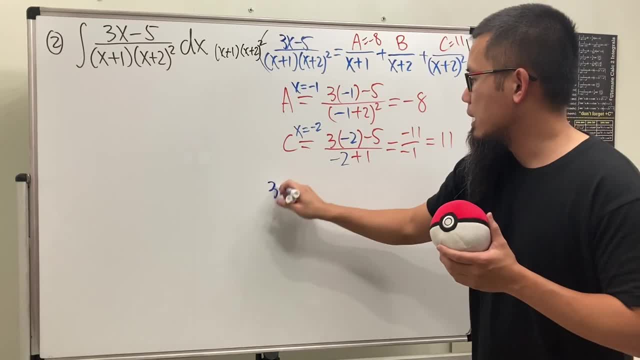 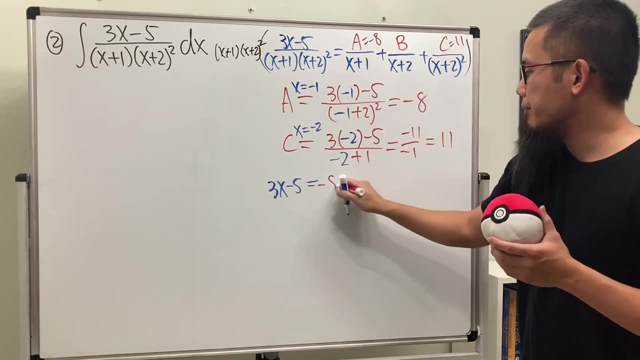 the numerator, which is the 3x minus 5. And then when we do this times that the x plus 1 cancel, So we get the negative 8. And we will still have to multiply by this guy. So it's slightly longer for this question. So we 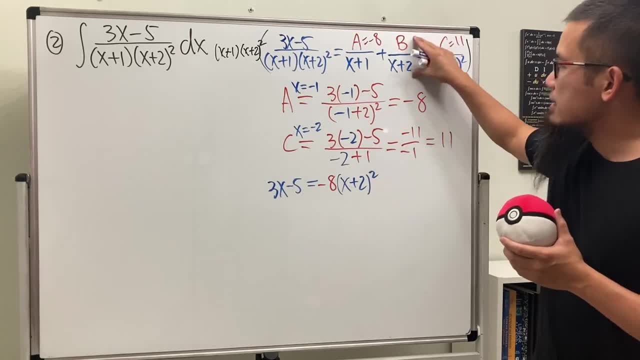 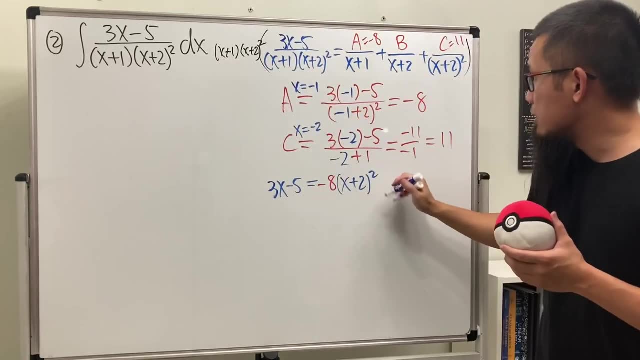 have x plus 2 squared And then this times that one of the x plus 2 cancel, So we will still have to have this, which is, let me just write down, plus b, And we get this right here first, So x. 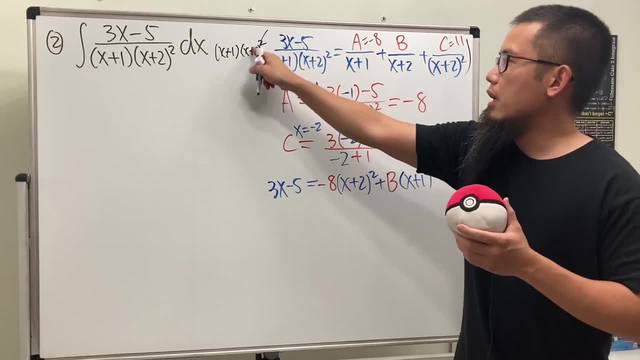 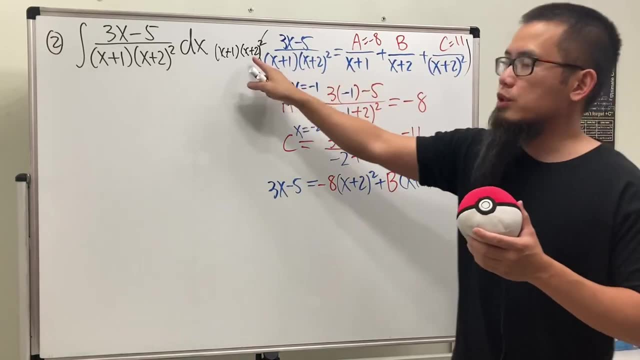 plus 1.. And we still have to multiply by another x plus 2, right, Okay. And then, lastly, we do this times that the x plus 2 squared cancel, So we just have the c, which is plus the 11.. 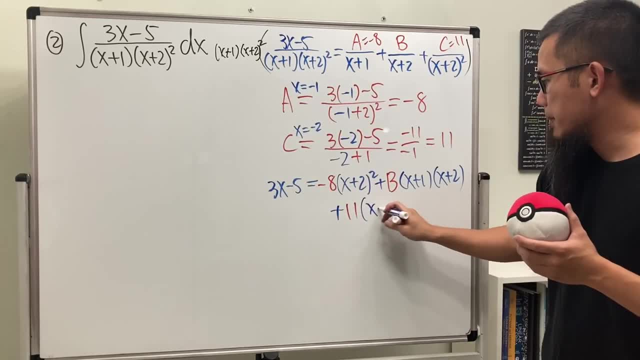 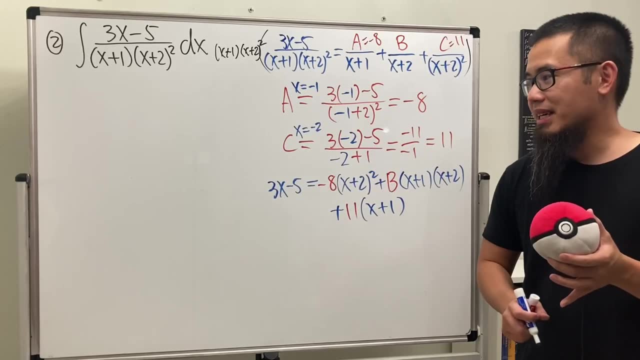 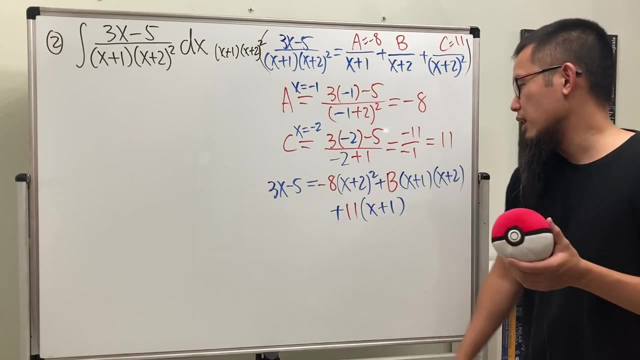 And we have the x plus 1.. Yeah, You can just go ahead and multiply it out and solve this, Or you can also let x equal 0 and then just try to figure it out. But I want to be consistent, So I will just multiply this out, I think. 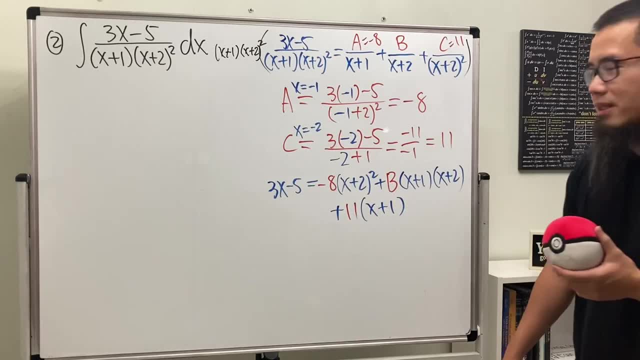 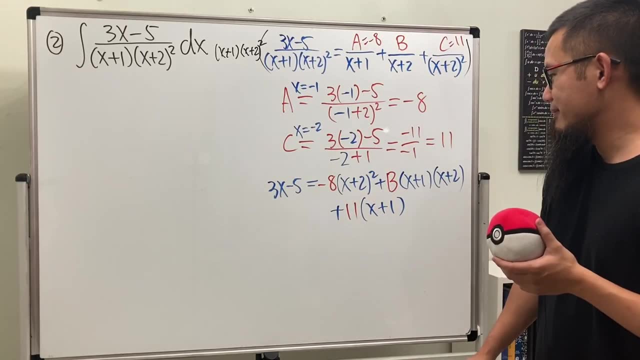 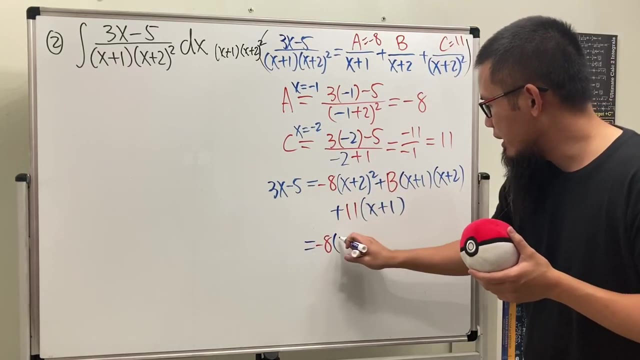 From my experience, you guys can follow along this way better. I know, it's just a lot of algebra, That's all Yeah. So what are we looking at? This right here is equal to negative 8.. And then this right here: when we open it, we get x squared plus 4x plus 4.. And then let's multiply this out. 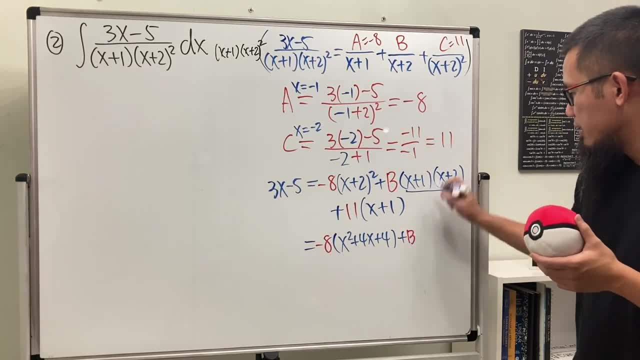 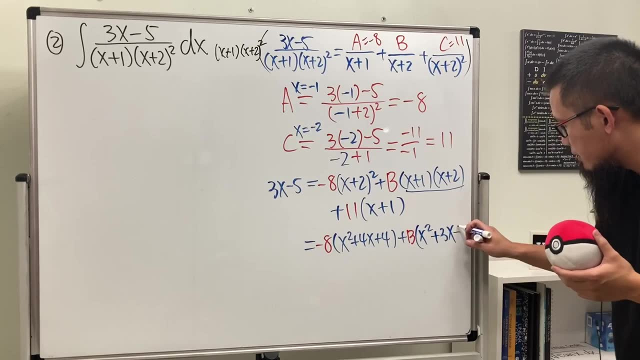 first: Yeah, So we get plus b. And then this right here is going to give us x squared plus 2x Plus x, So that's plus 3x, And then plus 2.. And then, of course, for this guy we can just: 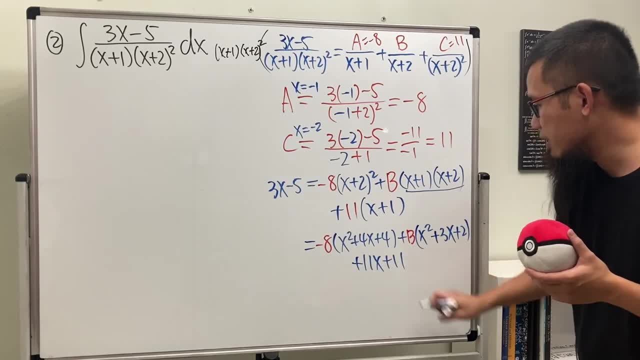 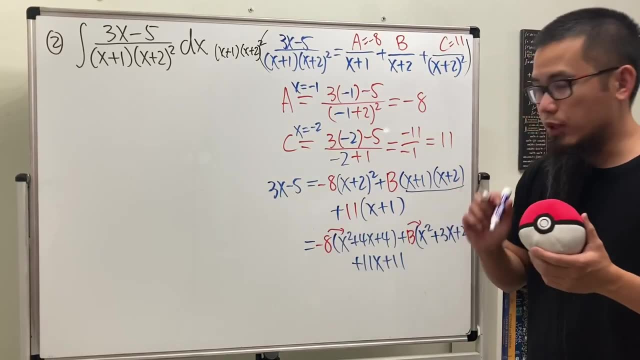 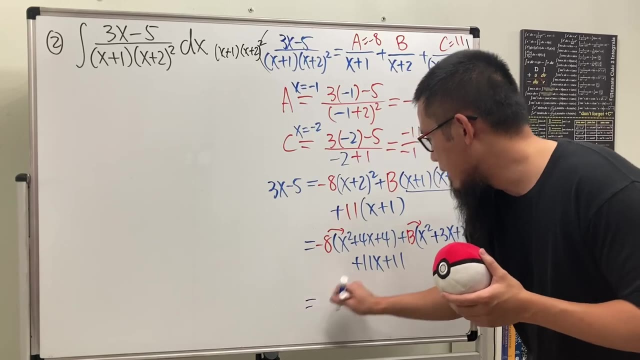 distribute, So we get plus 11x, plus 11.. And right here we just distribute. But in fact we just need to worry about this and also that. And the reason is because they will produce the x squared term right, So we will look at negative 8x squared. So let's look at it like this: And then 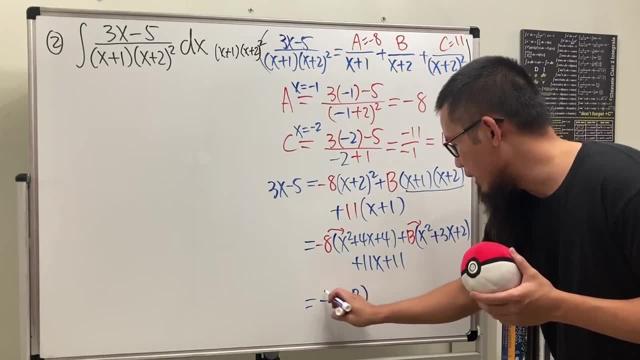 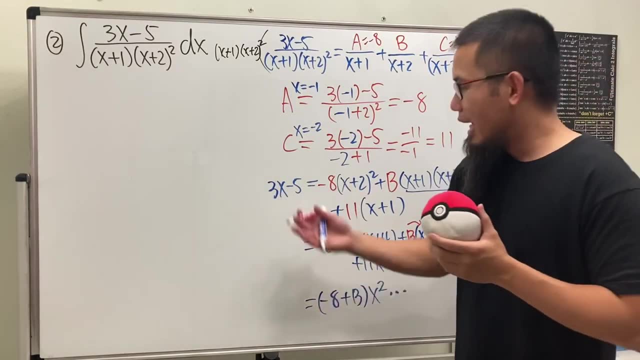 bx squared, So I'll just put on plus b And then we have the x squared term And again we don't really need to worry about what's after that. And as we can see, on the left-hand side we do not have x squared, So that means we have 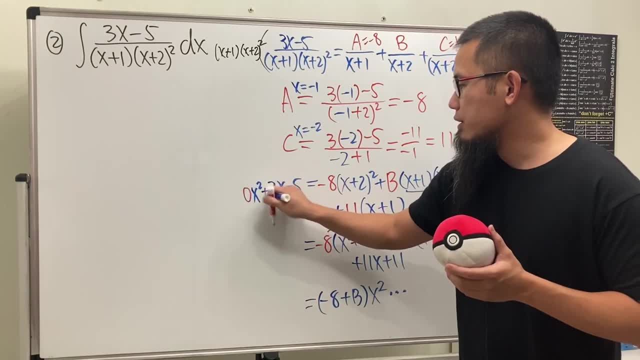 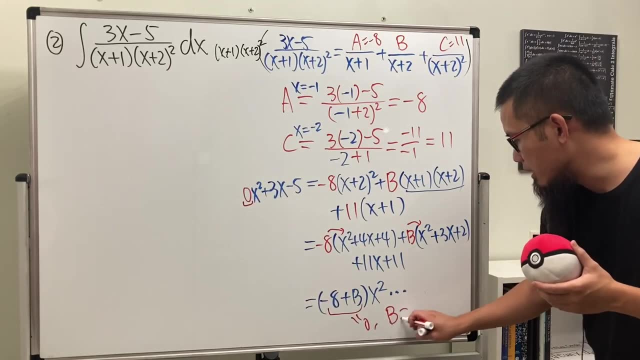 0x squared right. So that means 0 is for this. OK. So this guy has to be equal to 0. That means b has to be positive 8.. Oh my god, This is my b And this is my 8, right, So that's the idea. 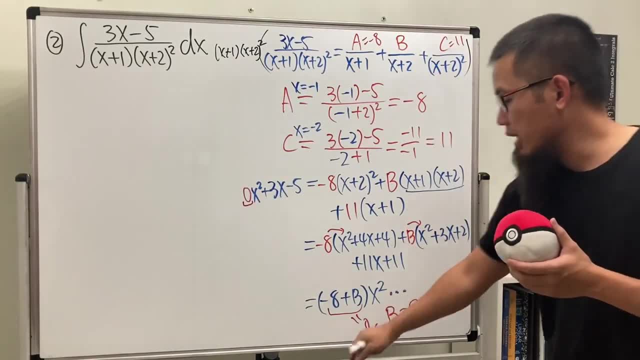 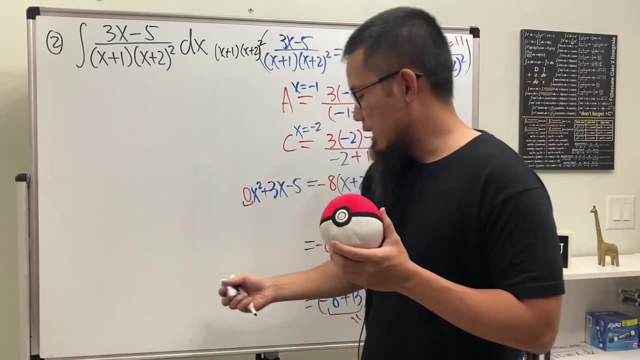 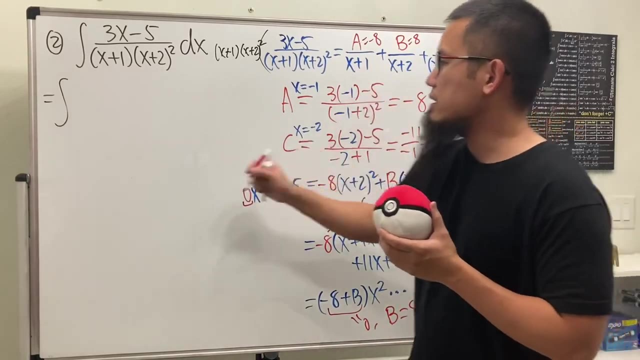 Cool. Now we can, of course, just do the usual business and finish this question, So let me just write this down. This is b equals 8.. Ladies and gentlemen, let's come back here. We have the integral right here, And the first one is negative 8 over that, So let me just write that down. 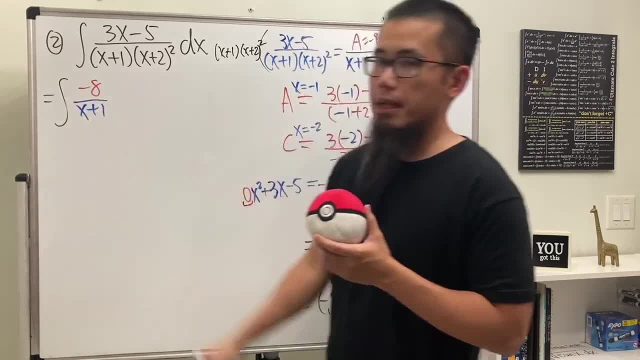 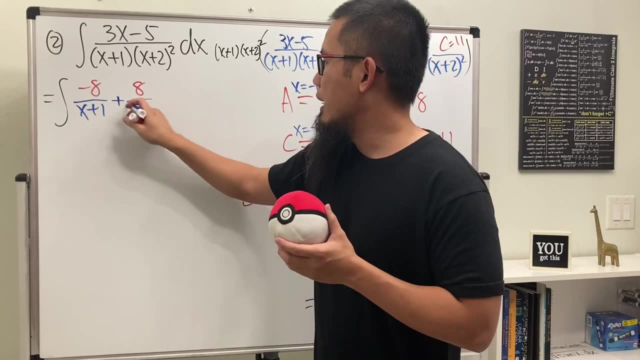 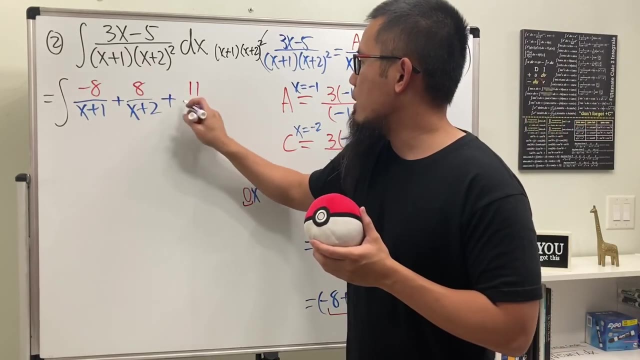 Negative 8 over x plus 1.. Next we have positive 8 over that, So plus 8 over x plus 2.. And lastly we have 11 over that, So plus 11 over x plus 2, but to the second power And 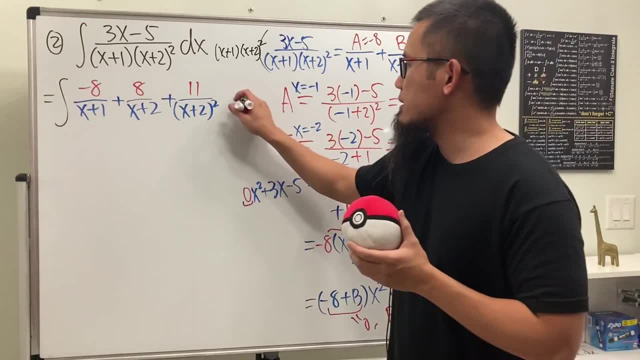 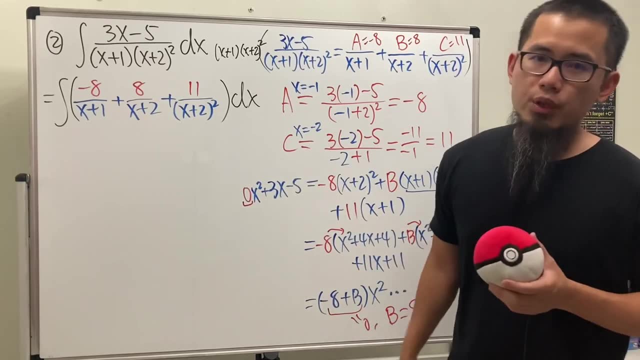 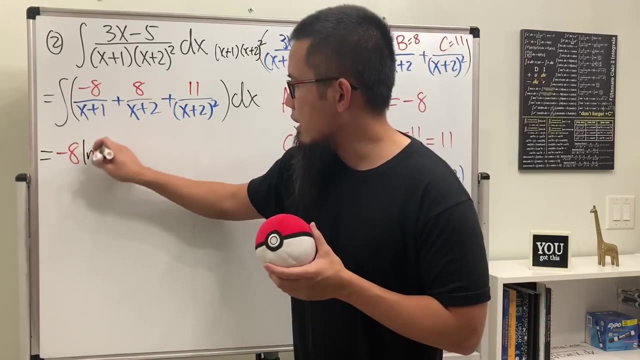 then right here we'll just close the integral with the dx And again, let me just put down parentheses to make people happier. But yeah, we're ready to integrate. For the first one, that's a constant multiple. On the bottom we have a linear factor, So that will give us ln. 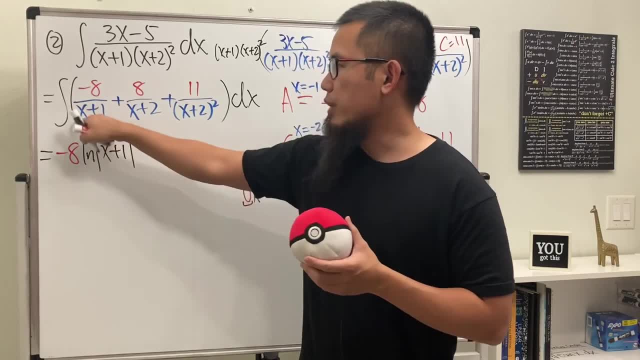 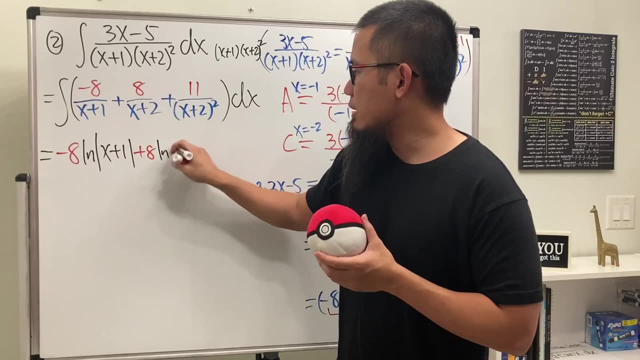 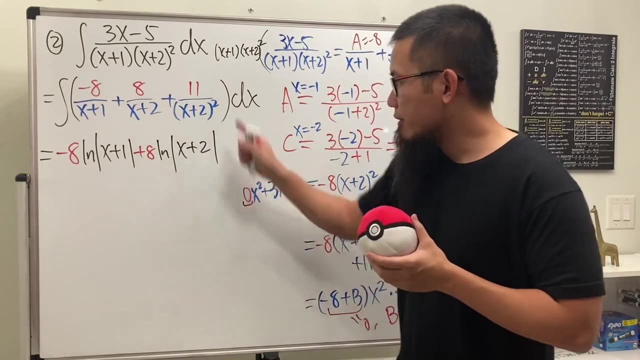 absolute value Of this, And the coefficient right here is 1.. So we didn't have to define anything. Continue. Next one positive 8.. So plus 8.. And then ln absolute value, x plus 2.. Now for this guy right here, we have the positive 11.. So I'll just put that down. 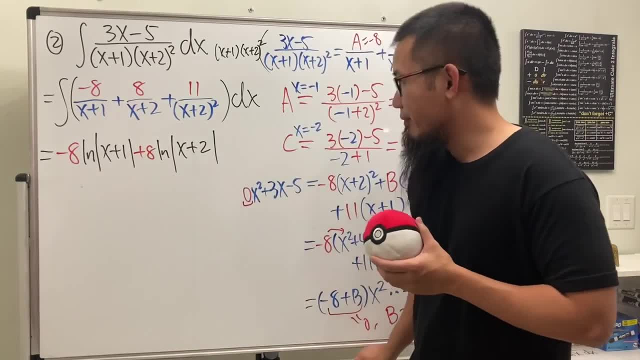 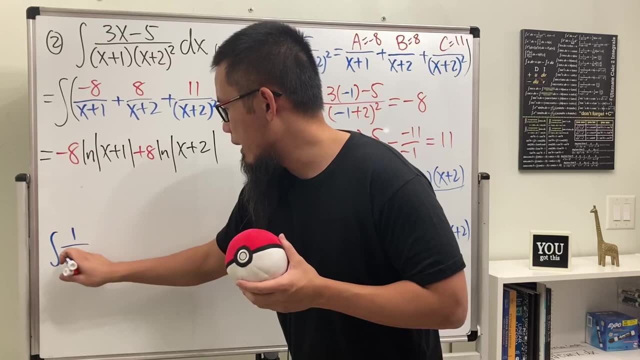 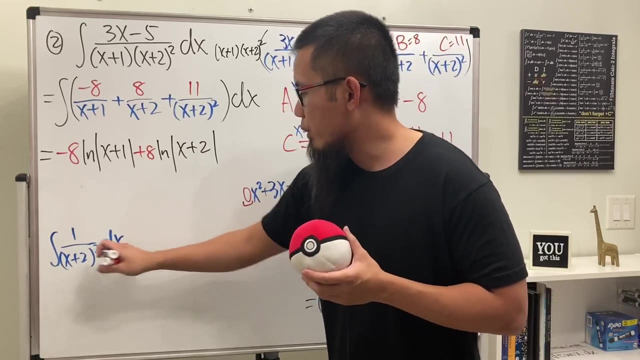 Actually not yet. Let me show you guys this: first We have the 11, right, And then we have that. Let's just focus on the integral of 1 over x, x plus 2 square. To integrate this, we do u sub, Let u equal the denominator, which is x plus 2.. 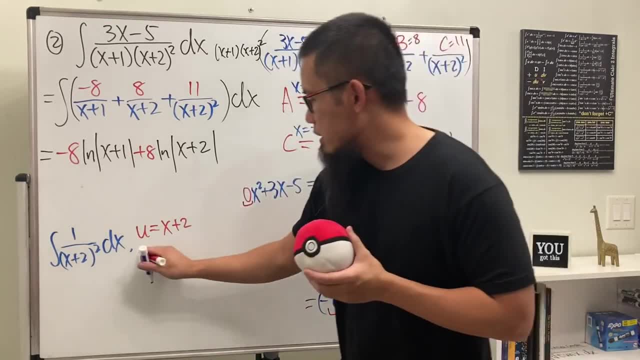 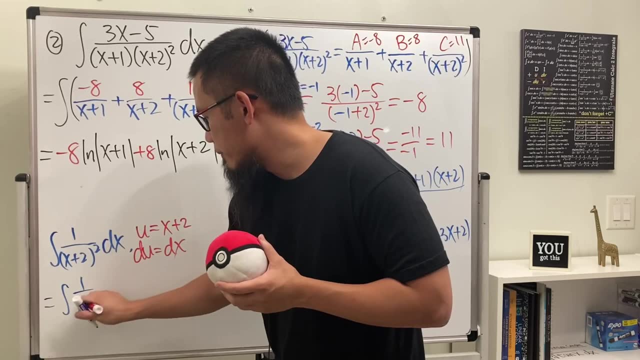 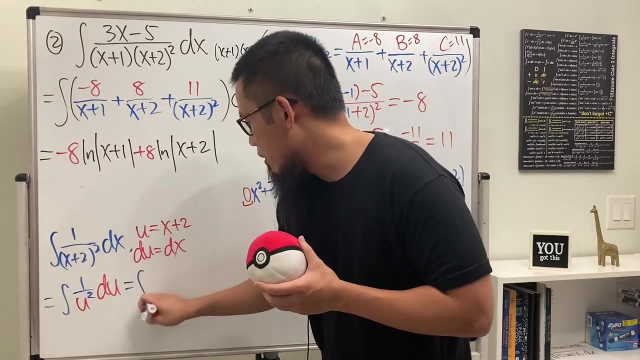 Actually just the inside. We don't want it to be the second power And we'll see this is just du equals dx. And we see this is just going to be integral 1 over u square du. This, right here, means we get the integral of u to the negative 2.. 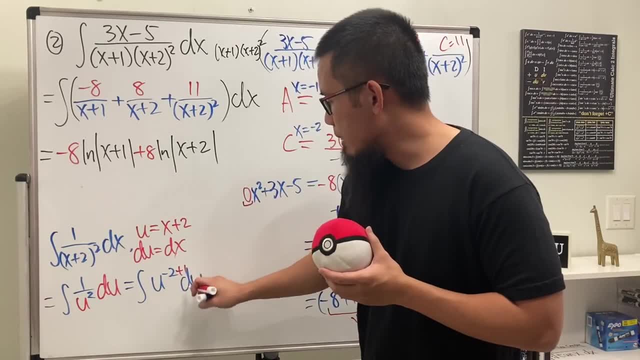 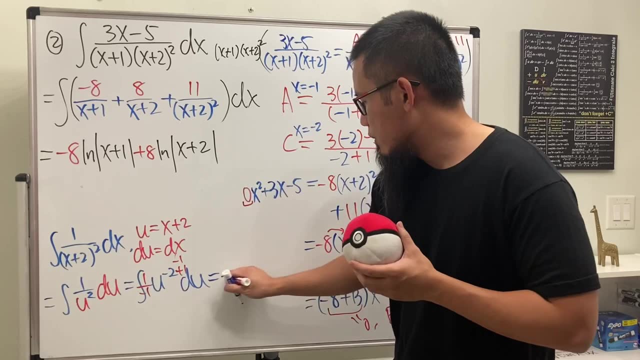 In the? u world. So integrate this: You add 1 to the power, We get negative 1.. And divide it by the new power, So we get negative 1 over u, because we have the u to the negative 1. And u is x plus 2,. 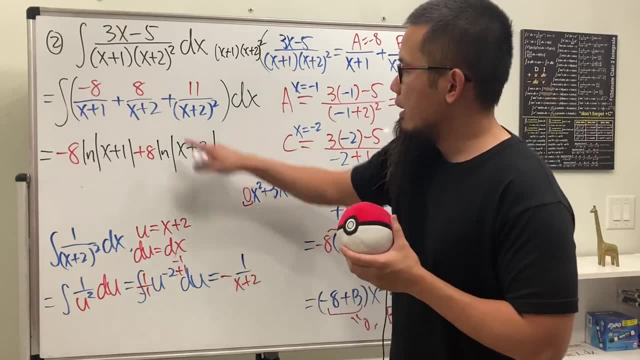 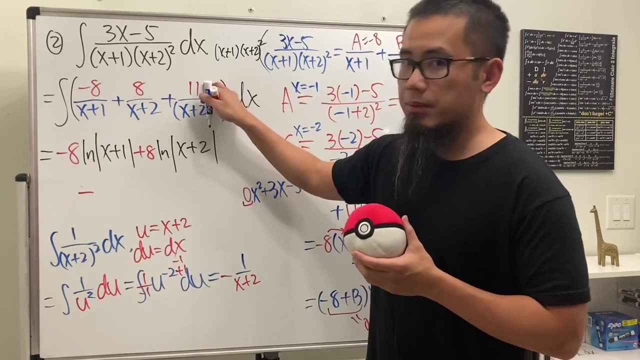 right, So we just put that down. Yeah, Anyway, earlier it was plus, But right here it's a minus. So we actually have a minus here, And then we have the constant multiple 11. So let me just put that down here. 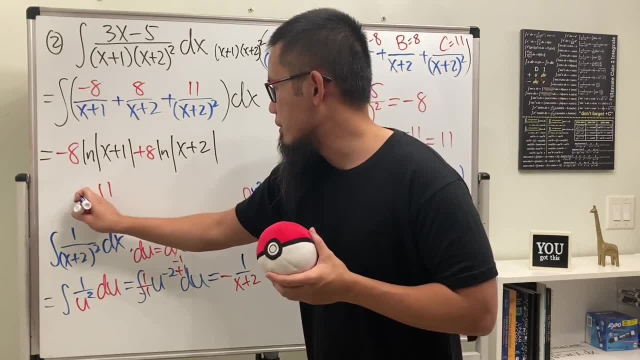 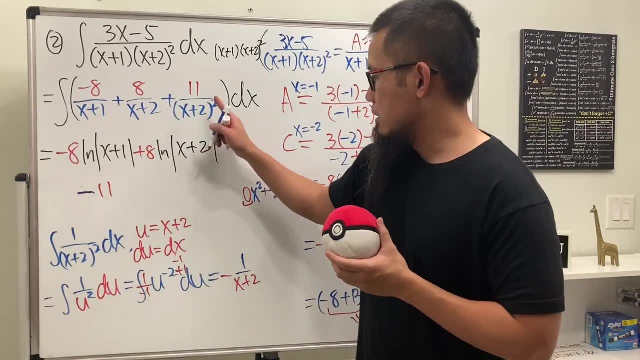 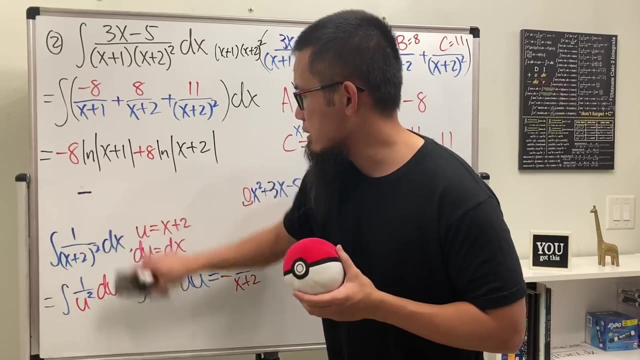 And let me just put down this in blue: Yeah, because we integrate this right, That's the negative integral right here, And we have the over x plus 2.. So over x plus 2.. Yeah, So just like this. So perhaps I'll just write it down slightly better for you guys: Minus 11 over x. 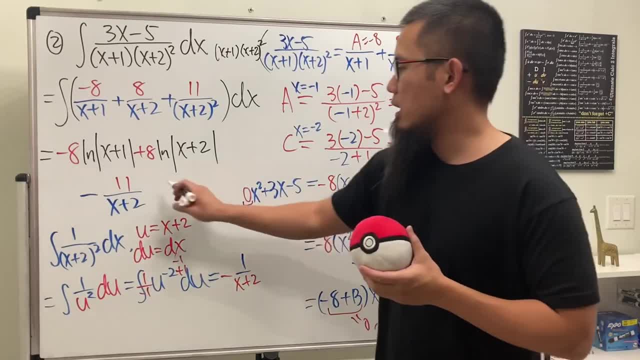 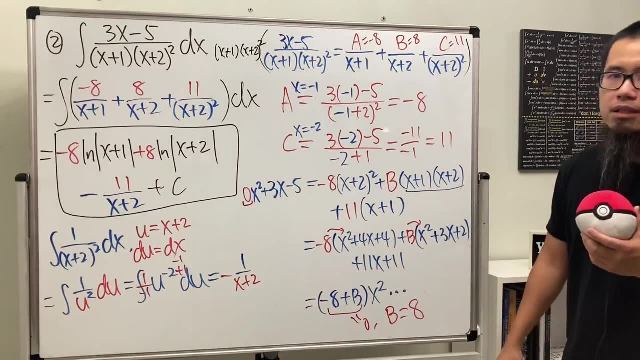 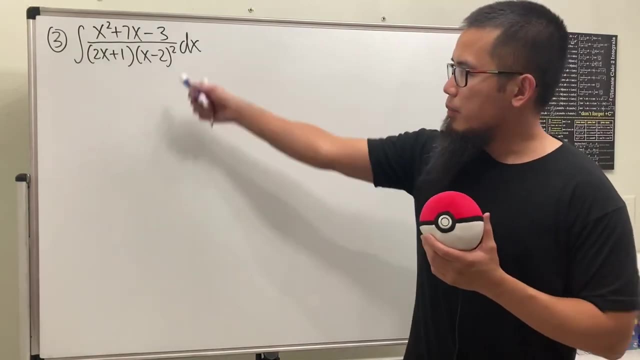 plus 2.. Okay, And we're all done After we put down the plus c. this right here. you'll see it right here. Yeah, So take a look at all this. All right, Number 3 right here. And okay, Number 3. 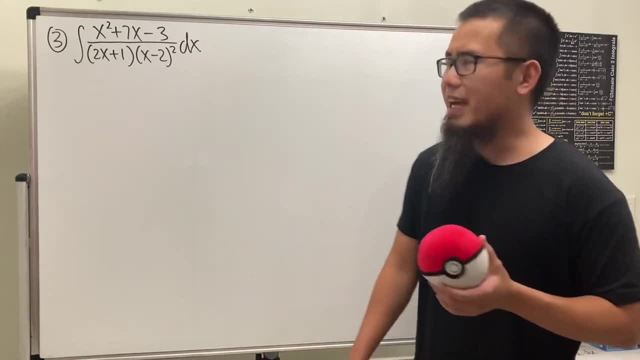 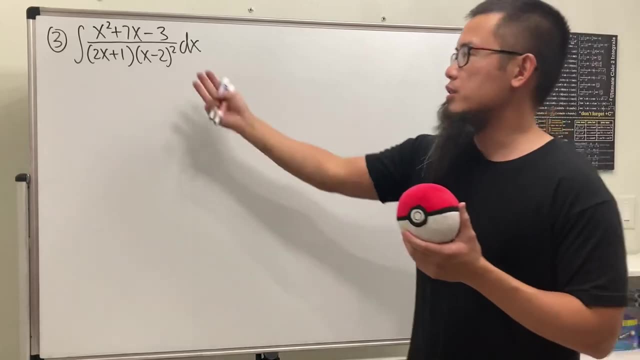 here Again the denominator has been factored in for us, which is very nice. On the top degree is 2.. On the bottom degree is 2 here and 1 here. So when you multiply you add the exponent, So the. 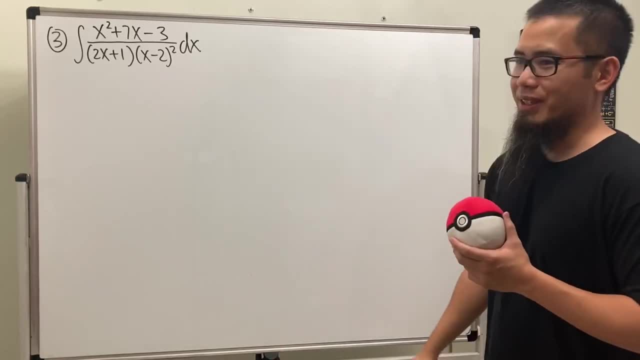 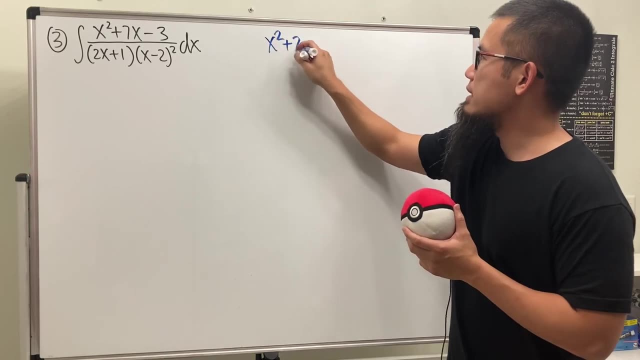 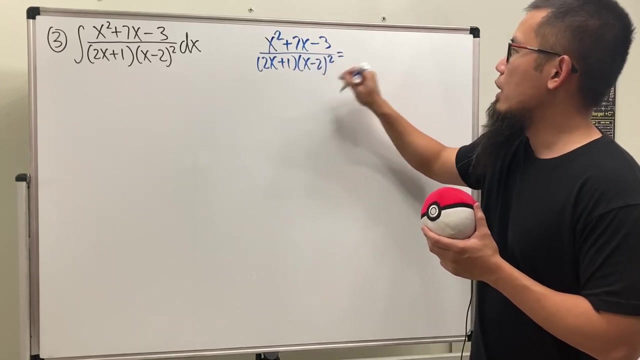 degree is 3.. We don't need to do long division, But we still have to do the partial fraction, Okay, So let's go ahead and work that out right here. So let me just write that down Again: x squared plus 7x minus 3 over 2x plus 1 times x minus 2 squared. Well, this right here. 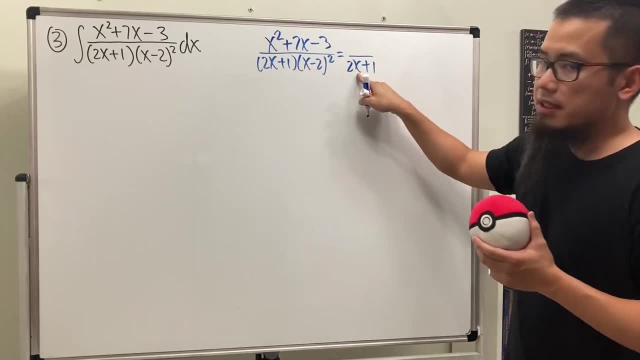 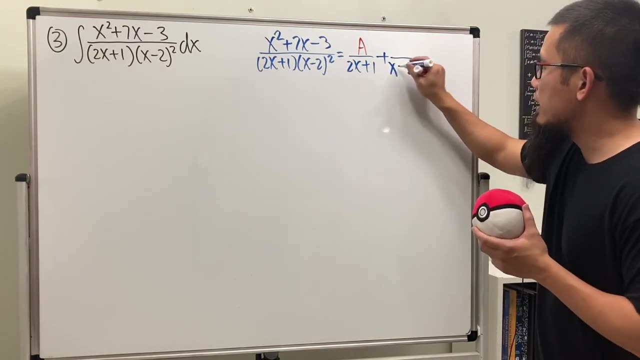 will be going first right: 2x plus 1.. Because this linear on the top is just going to be constant. And then we add: Here we will have to build up the power. So we start with x minus 2 here. 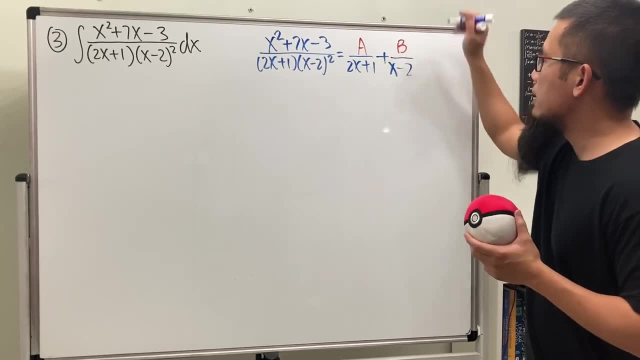 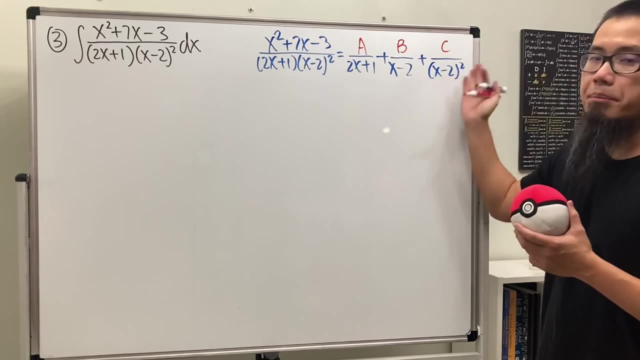 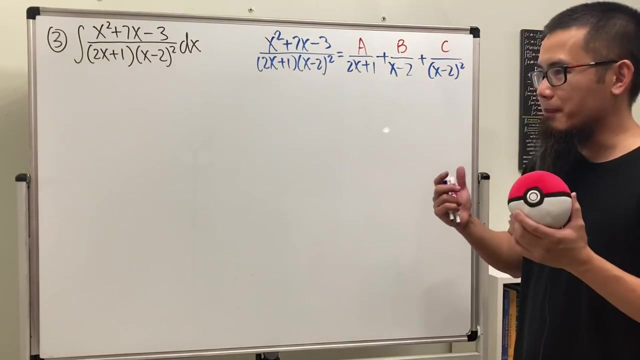 to the first power On the top. it will be a constant. And then, right here, we will have the x minus 2 squared On the top. we will still be a constant because we are building up the power. All right. Again good news: We can solve two letters by using the. 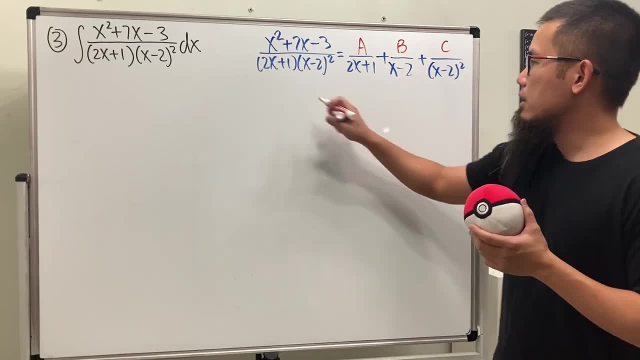 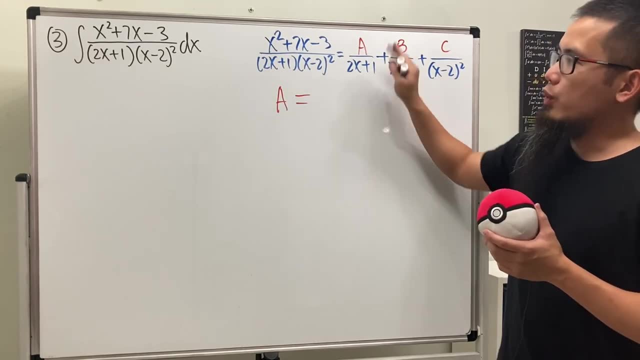 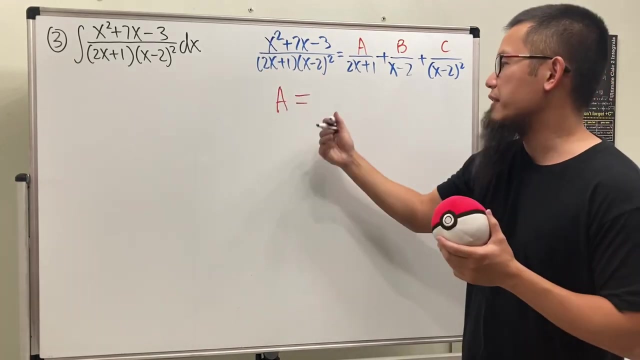 copra method, And that will be a and c For a. well, this time slightly trickier, Because the denominator is 2x plus 1, we come here and we copy this up: How can we make 2x plus 1 equal 0? x has to be negative 1 half, So x is equal to. 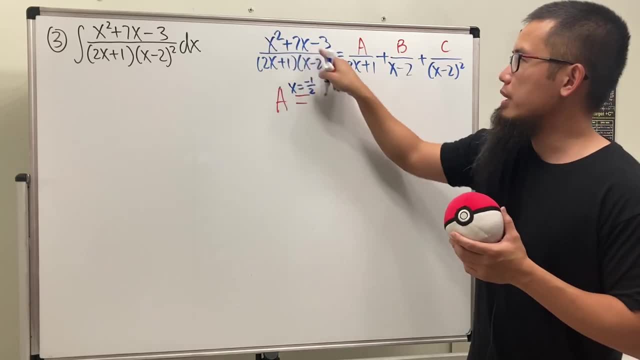 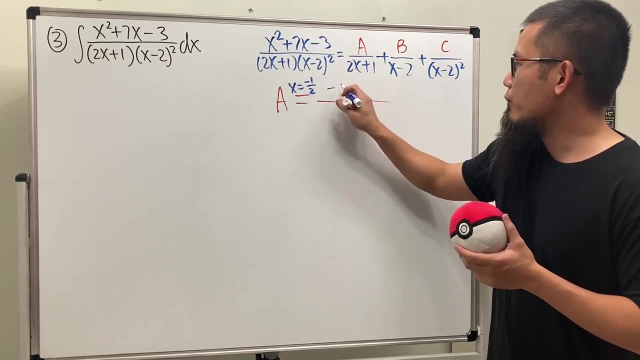 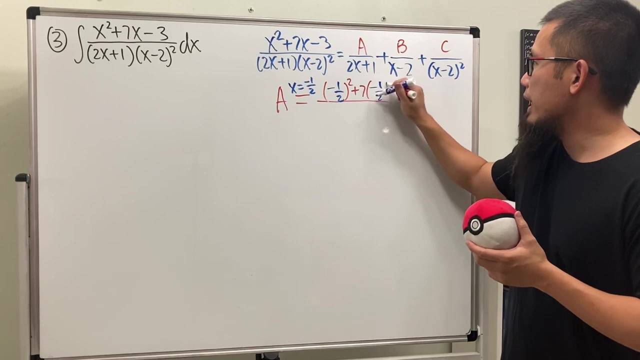 negative 1 half And we will just have to plug this in into all the x's and just deal with fractions. I know, OK, let's see if we can handle that. Right here we have negative 1 over 2 squared, And then plus 7 times negative 1 over 2 and then minus 3 over this right here is negative. 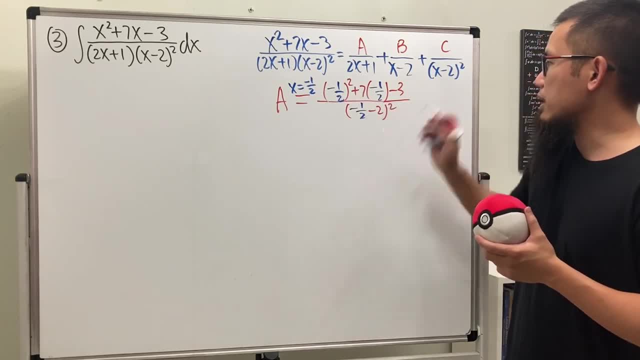 1 over 2 and then minus 2, and then to the second power. All right. So let's see, This is going to give us Positive 1 over 4.. And this is going to give us negative 7 over 2 and then minus 3.. And on the 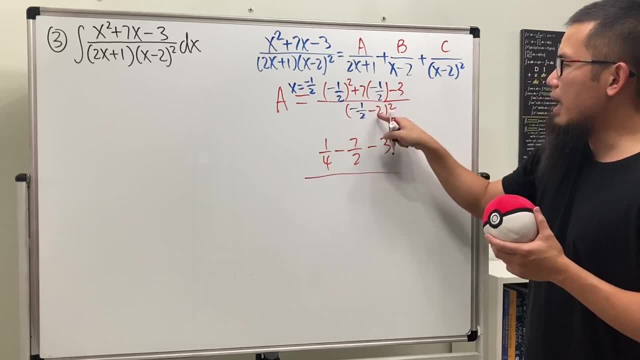 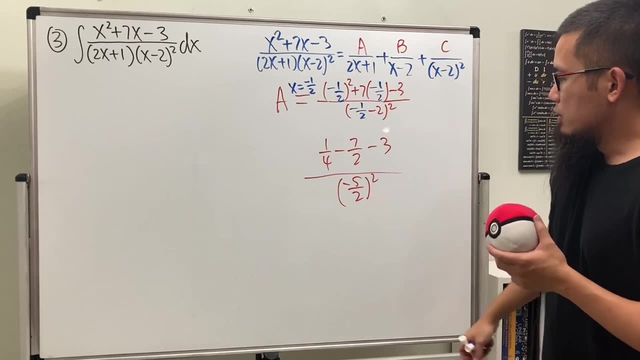 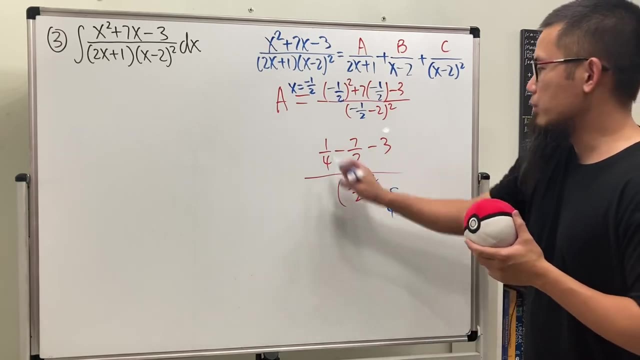 bottom. this is going to give us negative 5 over 2.. Right, Because you just get a common denominator all worked out And then you have to square that. So when you square that, this is just the same as 25 over 4.. So what we can do is just multiply the top and bottom by 4.. Why? Because this way. 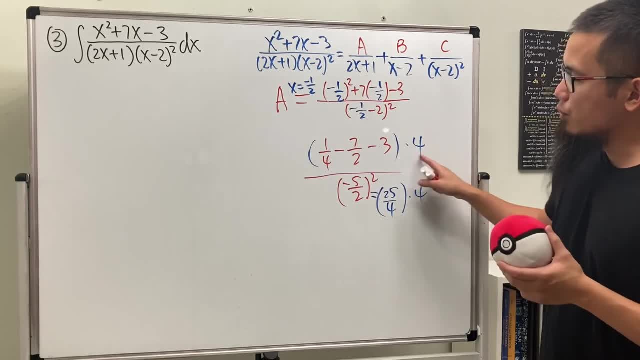 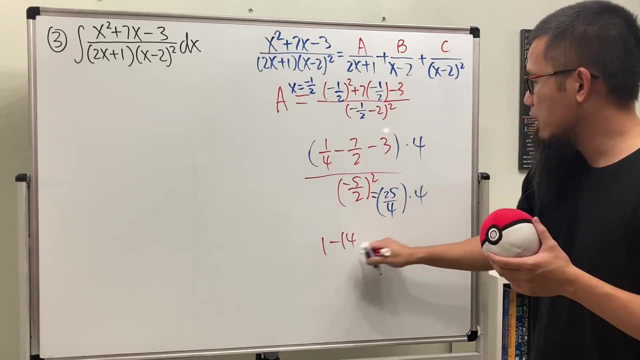 we can just get rid of the complex fractions. I think it's easier that way. So if you do this times that we get 1, minus this times that reduce it, You have 2 times, that is 14.. This times that. 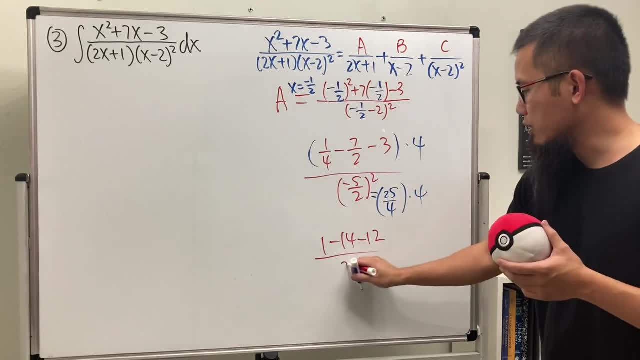 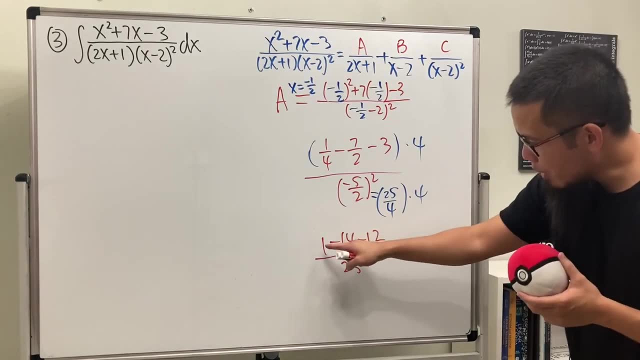 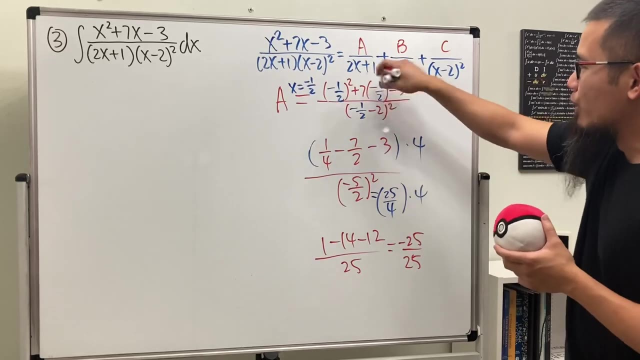 is 12 over this times that we just get 25.. OK, let's see This: minus that is negative, 26 plus 1 is negative, 25 over 25.. Hey, what do we have? Yeah, Work this out. 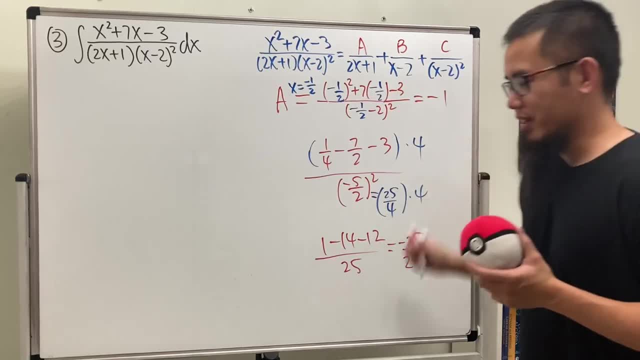 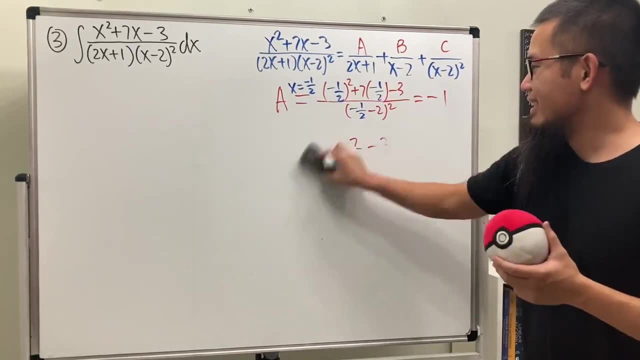 We'll end up with negative 1.. I know All the work for negative 1.. Yeah, but it's just arithmetic, So not so bad right. Not so bad, All right, Continue. We use the cover-up method for C. 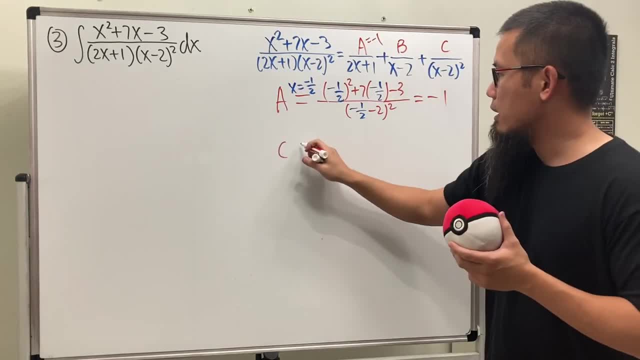 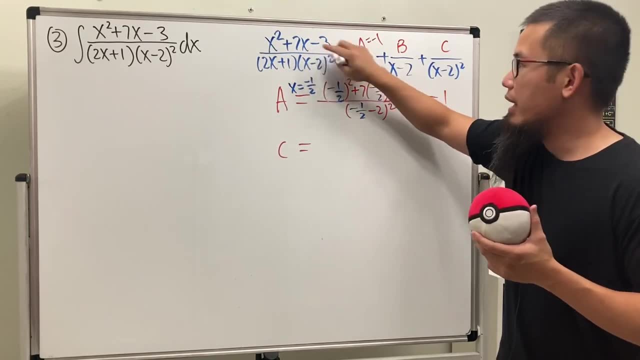 Right. AO is negative, 1.. C is going to be the following: We go back to the original. cover this up. And how can we make? X minus 2? squared equals zero. X has to be 2.. So let me even out that. 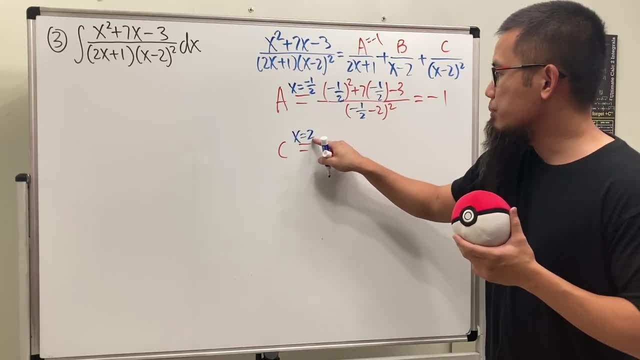 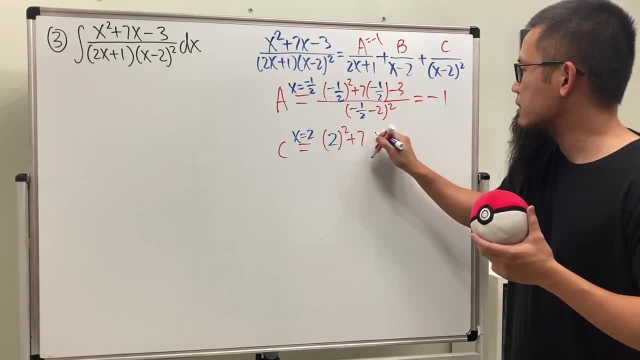 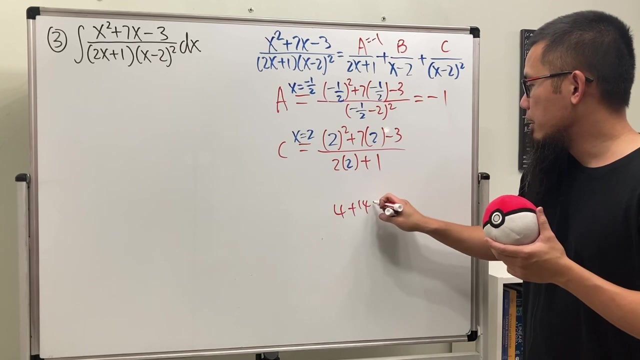 2 square plus 7 times 2, and then minus 3 over 2 here. so it's 2 times 2 and then plus 1. okay, okay, let's just work this out. this is 4 plus 14 minus 3 over 5, and this is 18 plus, so 18 minus. 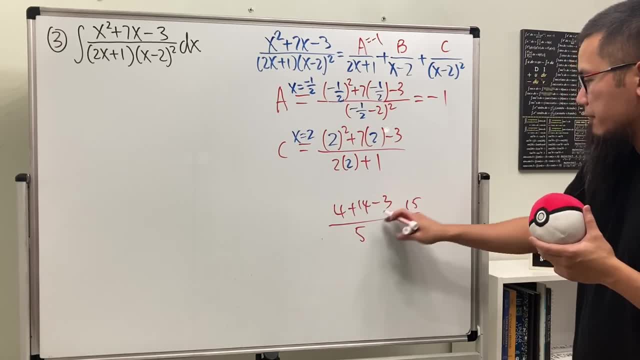 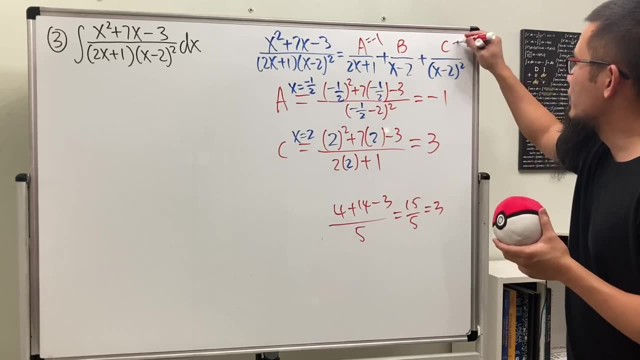 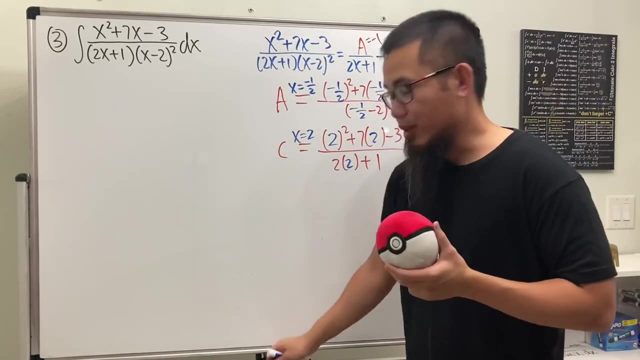 3 is 15 over 5, yes, and then this is going to give us positive 3, so c is also really nice. so here we have. c equals 3. all right, now for b. yeah, we just have to do it the good, old-fashioned way. 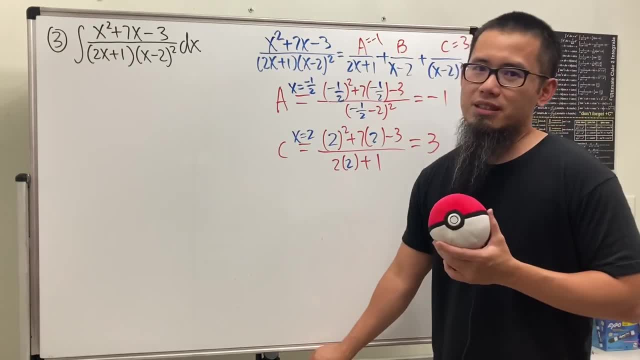 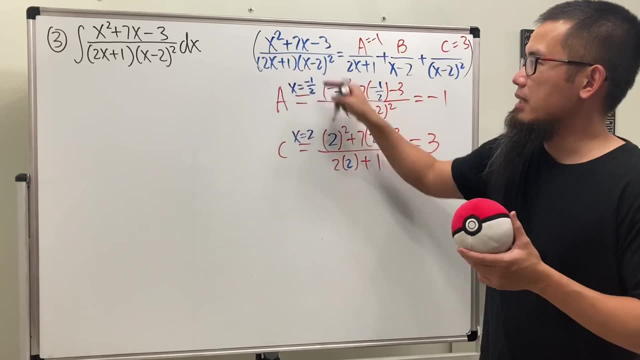 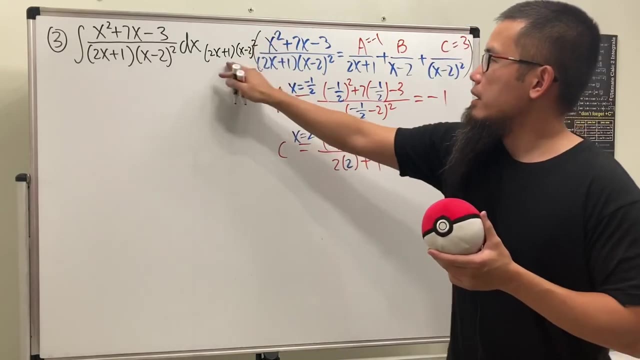 so, so, uh, again, it's just because i think it's more consistent, it's more clear for the students, for you guys. so yeah, let's multiply everybody by the common denominator, which is just that. so let me put down 2x plus 1, x minus 2, square, this times that we'll just have the top right here. 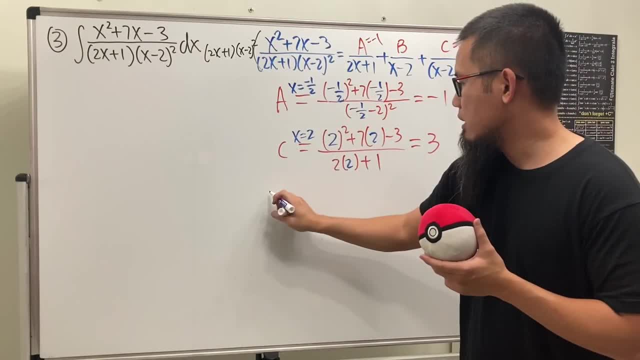 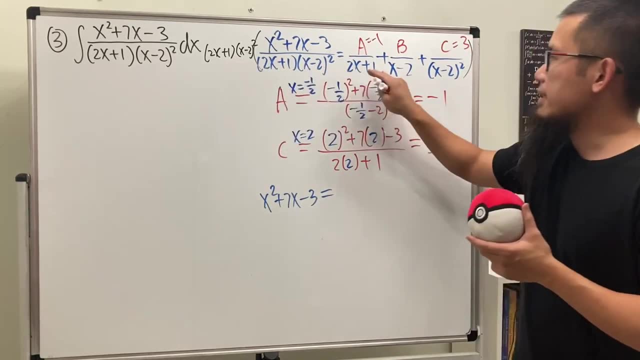 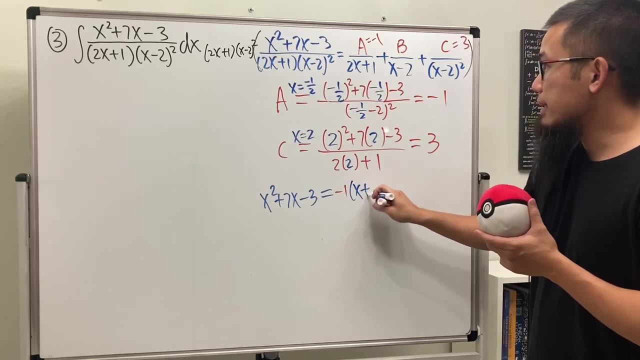 so let's look at here: x square plus 7x minus 3, that will be equal to this times that the 2x plus 1 will cancel. so we have negative 1 times this, which is x plus so x minus. so be really careful. 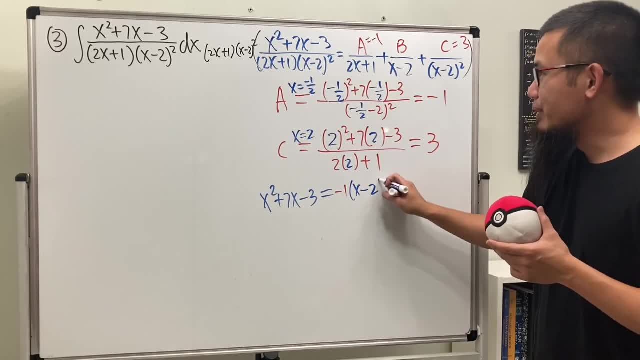 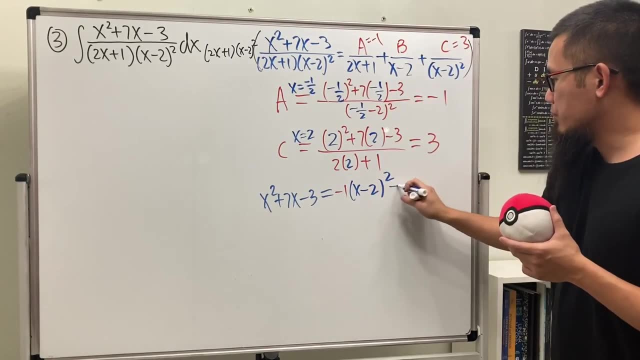 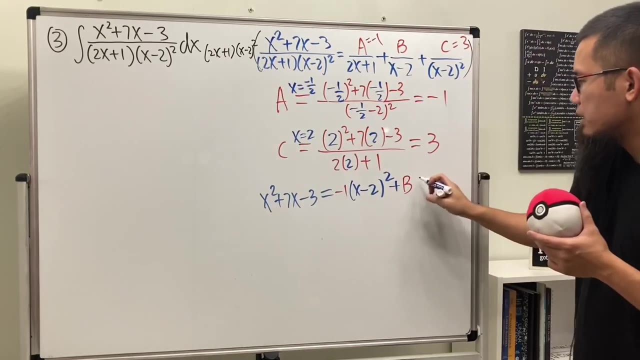 you see, yeah, x minus 2 square. i make mistakes too, so just be really careful. for that, all right. and then for the next one, b, we don't know. so put down plus b and then one of them cancel out, so we will have this and that. so b times 2x plus 1 and then x minus 2 square, so we have negative 1 times this. 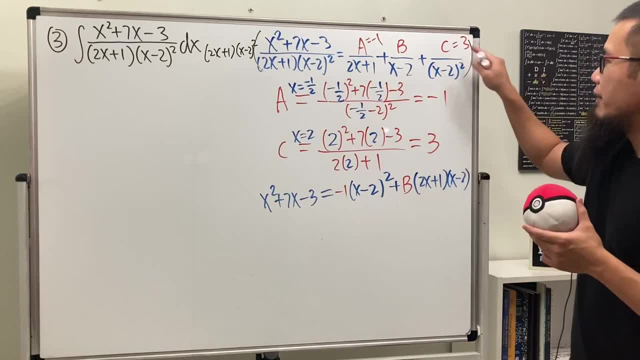 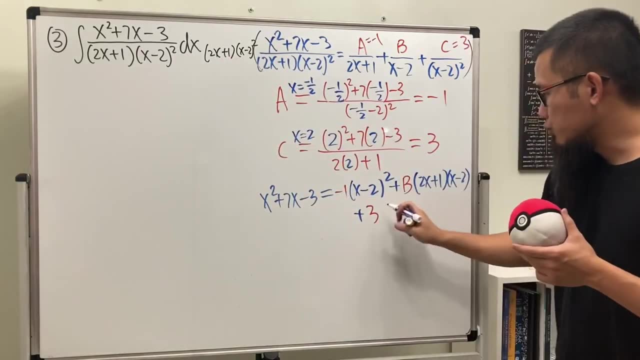 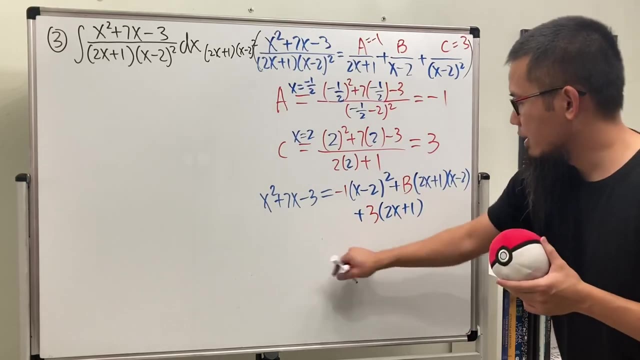 x minus 2, and lastly we have the c, which is 3, this and that cancel. so we just have that right here. so 3 times 2x plus 1.. all right, so, uh, just work this out here, we will see. this is negative. 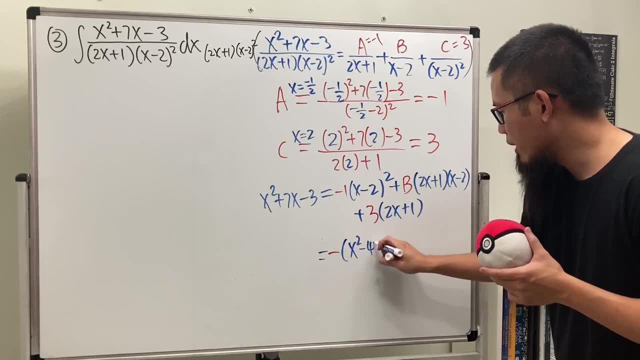 expand this, we get x square minus 4x plus 4, and again, let's multiply out the binomials right here, so we get x square minus 4x plus 4, and again, let's multiply out the binomials right here, so we get. 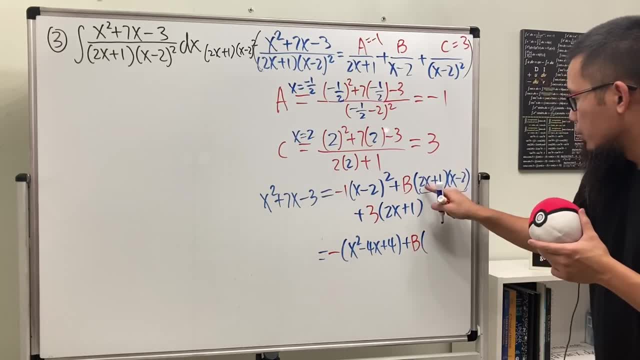 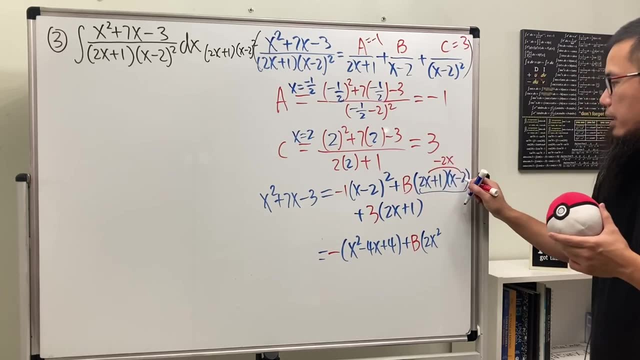 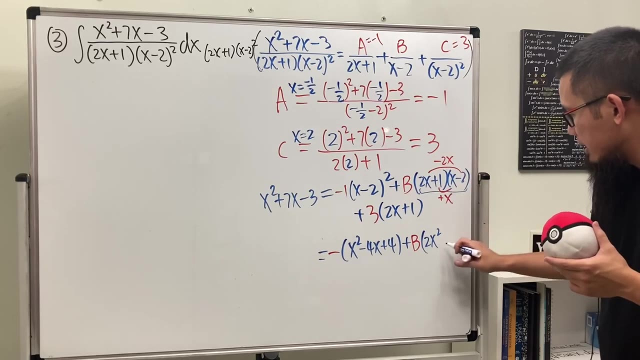 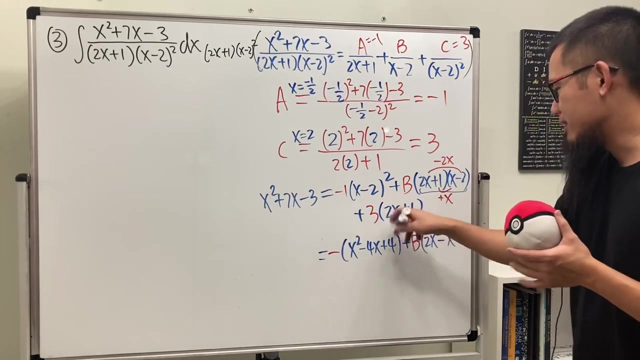 plus b, okay, 2x square, and then this is going to give us negative 2x and then minus, sorry, negative 2x and then plus x, so together we'll get negative x and then minus 2. right, when we do this times that, and of course, on the bottom in fact, it doesn't really matter. it doesn't really matter about. 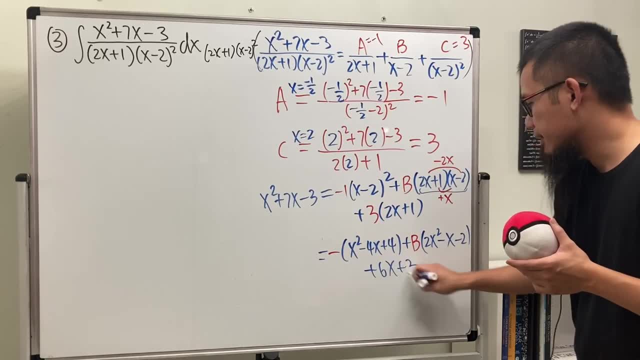 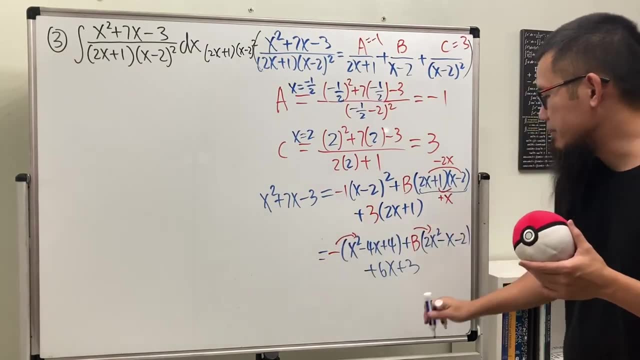 multiply down anyway, plus 6x, plus 3.. but it doesn't really matter why. it really matters is the coefficient of x squared right again, just like what happened earlier. so we see this times that we end up with negative 1, negative 1, and then 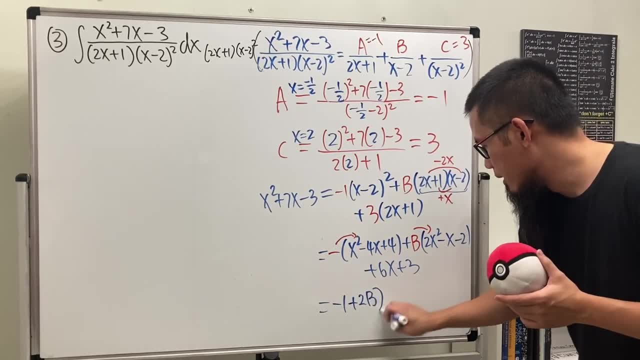 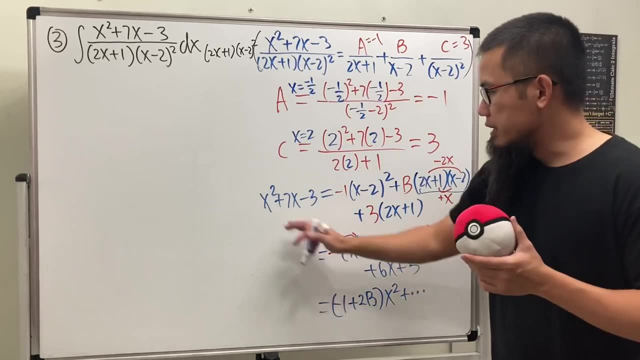 plus 2 b times x, squared and then, seriously, red rest. we really don't care. well, you see, on the left-hand side this time the coefficient is one. right, the coefficient here is one now, by the way, you can also compare the third part here. you can see that, by the way, we did this again, by the way. 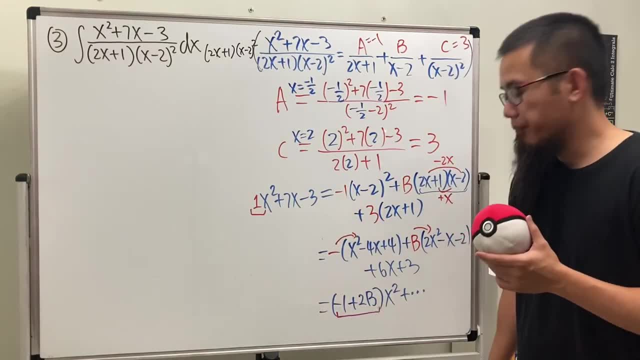 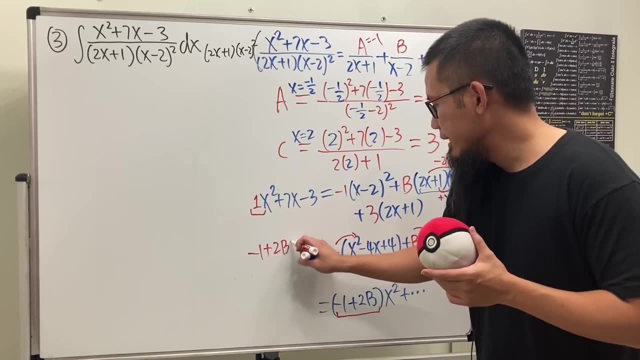 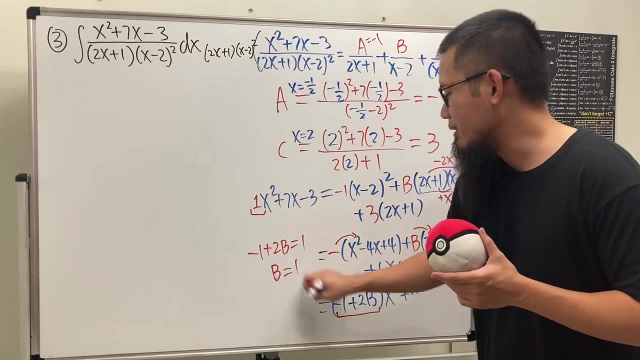 coefficient is 1 and the coefficient right here is this. so that means they must be equal. so we will look at negative 1 plus 2. B equals that which is 1. move this to the other side, which is 2, and you know what B is just equal to 1. 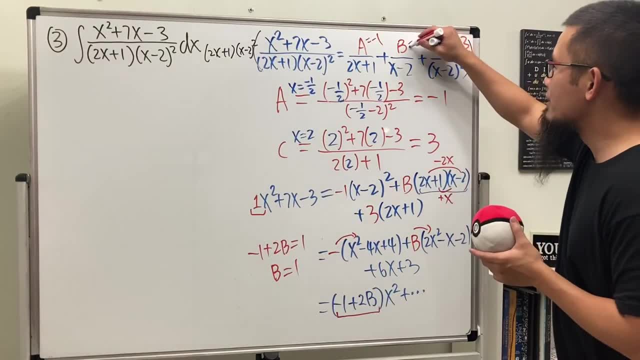 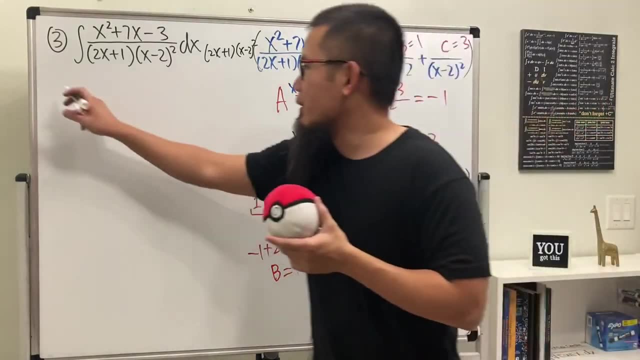 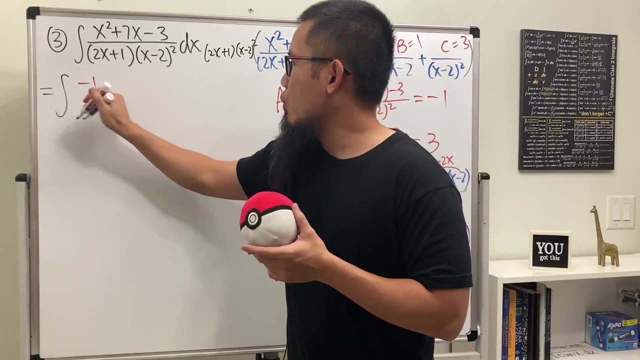 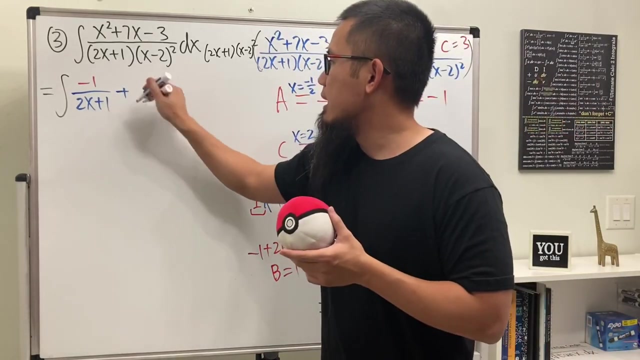 oh my god, all the work for B equals 1. yeah, all right, so now we go back there. and then we were just integrate. so here we go, look at the integral, and then first fraction is negative, 1 over 2x plus 1. next fraction, we have 1 over that. so we add 1 over x minus 2 and the next we 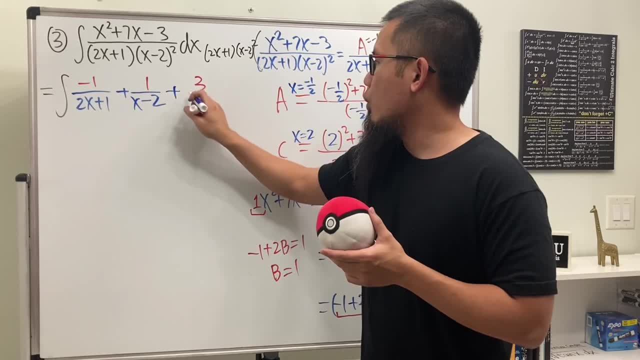 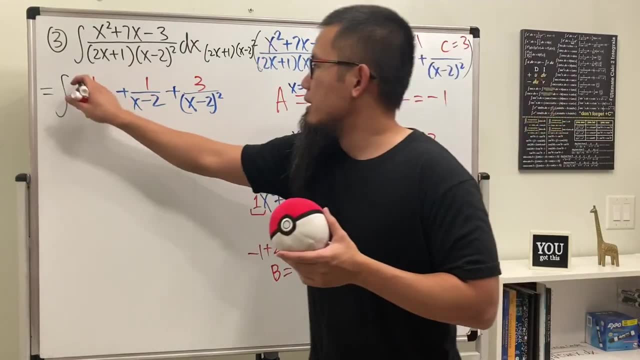 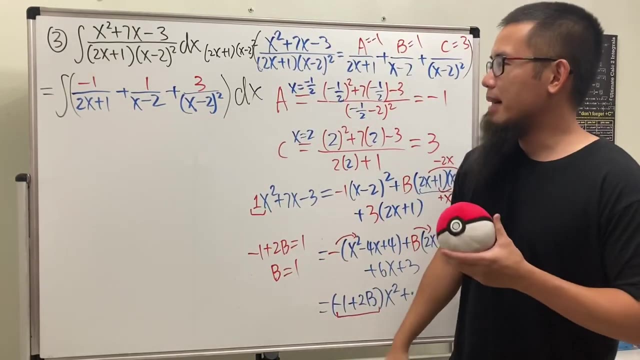 have 3 over that. so plus 3 over x, minus 2. but to the second power: yep, you know, of course, Just put on parentheses to make people happy and the DX if you don't have the parentheses right here. I'm cool with that, Yeah, but anyway. 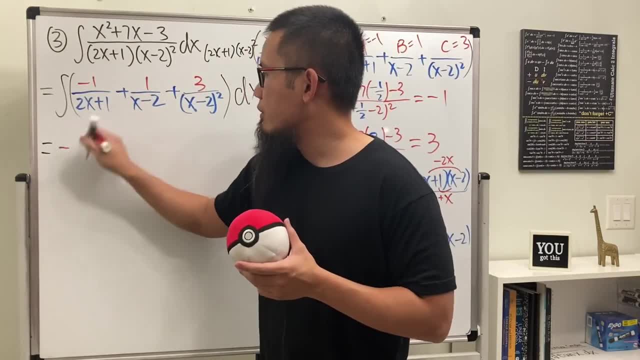 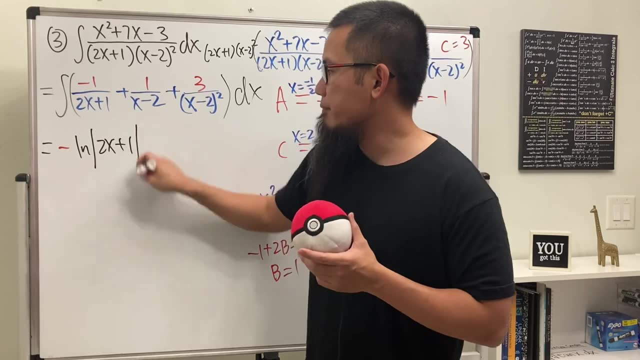 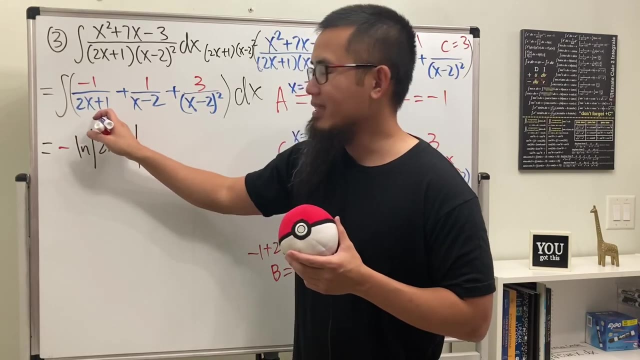 Here we go for the first one. we get negative Right and then on the bottom, linear, so we get LN absolute value of 2x plus 1. And what else do we need? Here we have the 2x plus 1, so we will actually have to divide it by 2. so just put down. 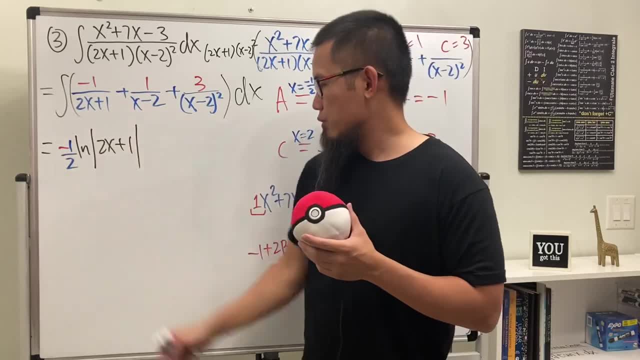 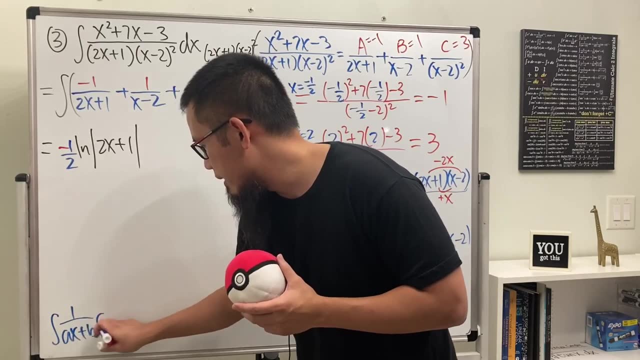 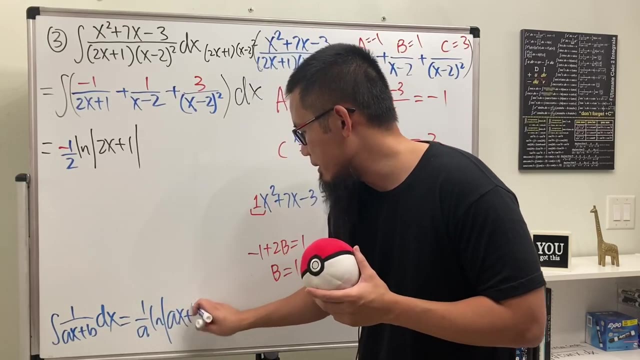 Negative, 1 over 2, like that. Remember, remember the formula, put it somewhere here real quick: when we have the integral of 1 over AX plus B, Right, this right here gives us 1 over a, now an absolute value of AX plus B. So that's why we are dividing by the 2. so that's what we have for the first part. 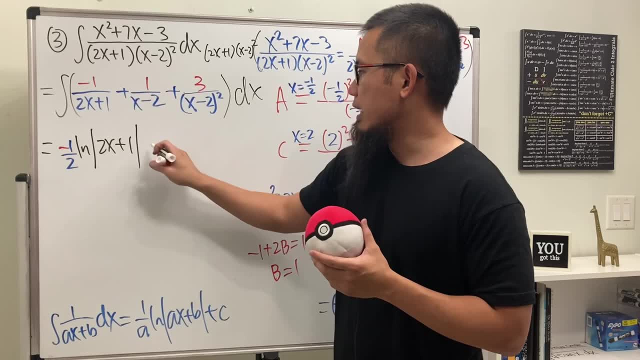 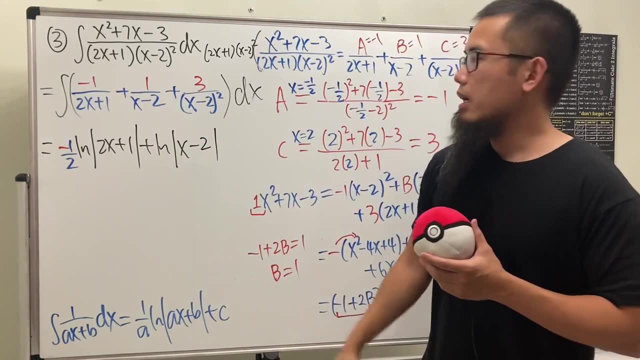 Next, this is just 1, so it doesn't really matter. I'll just say we add Ln of the bottom X minus 2 and the coefficient is 1, so doesn't matter. Lastly, we have the 3 over that, Which is very similar to what we did earlier. 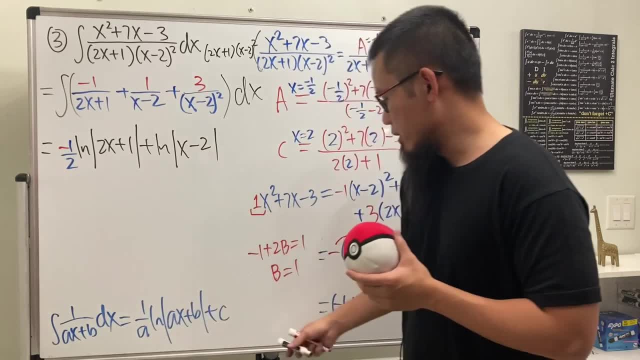 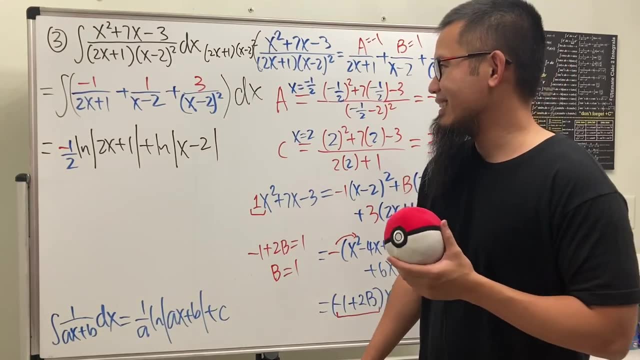 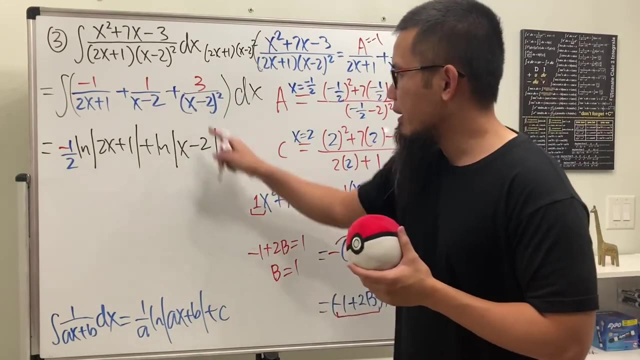 So I'm just going to do that again for you guys real quick, Alright, so well, actually you guys do it, Or should I do it? You should do it this right here. I'll just tell you: right, look at what we did earlier. When you do you stop, you end up with negative for the result, for the integral. 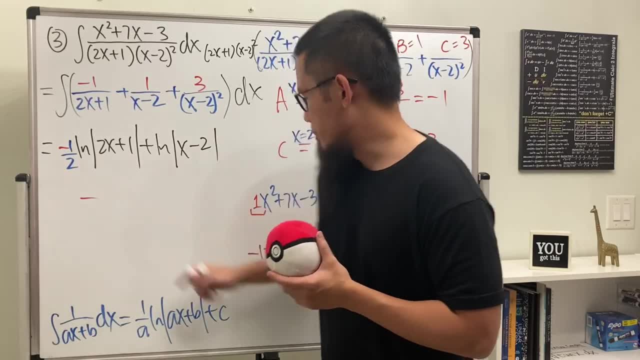 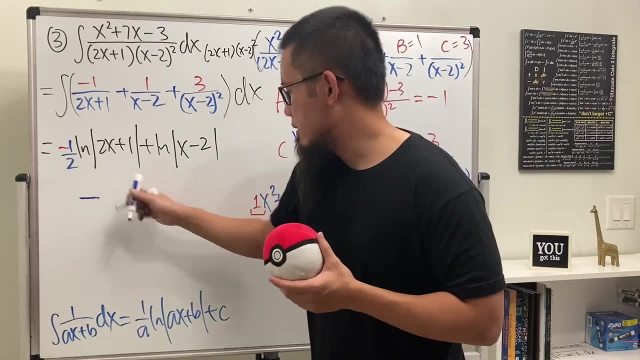 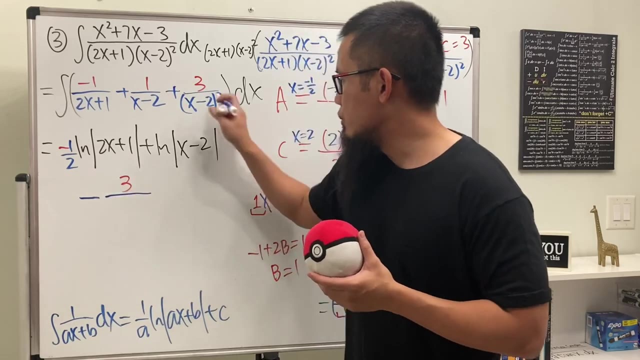 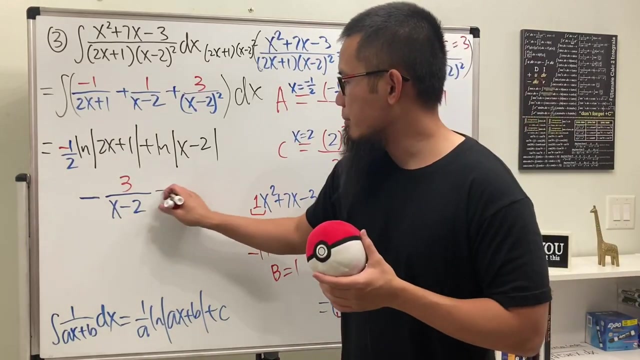 So it becomes negative. and then we have this 3, so perhaps the negative should be blue to make it more stand out. We have the negative, The 3, 3, The 3 over, Just X minus 2. All right, Very similar to what we did earlier. and we're all done. put on the plot. 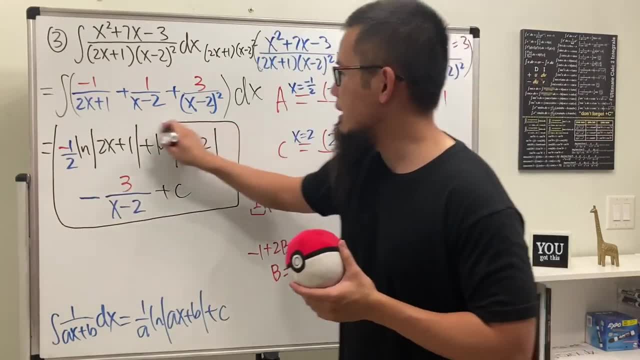 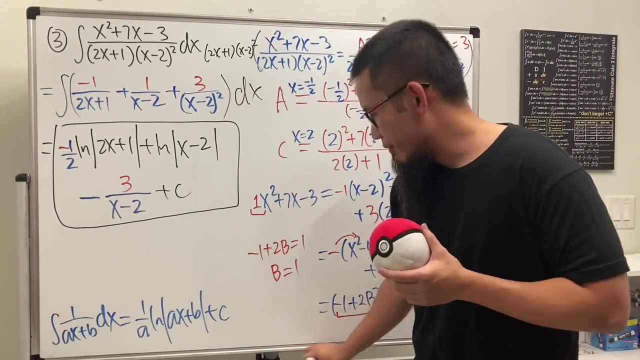 See, all right, so this right here is it. Huh, you want me to do it? Okay, I'll do it for you, this right here. Just look at the blue part. All right? so let me just do that for you guys real quick again. 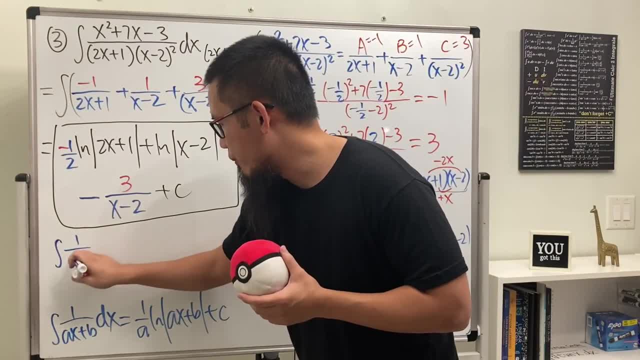 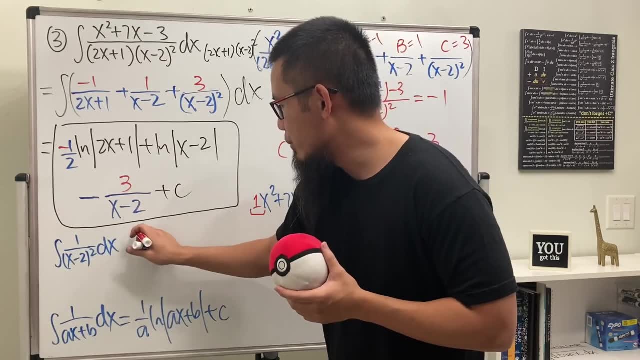 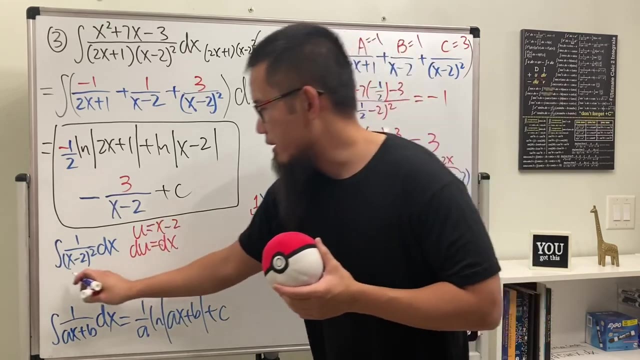 So when you have the integral of 1 over X minus 2 Square, You do the use up, you let you equal the inside here, which is X minus 2, and du is equal to DX. So this right here is just the integral of 1 over u. 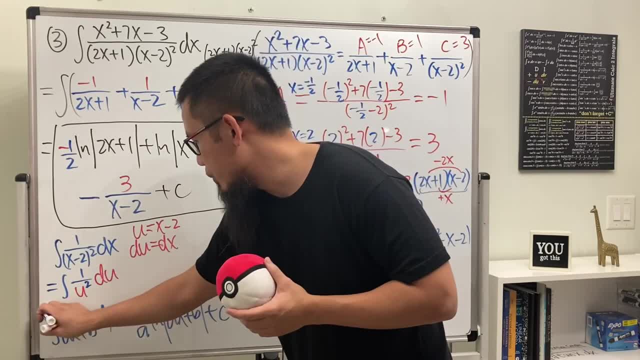 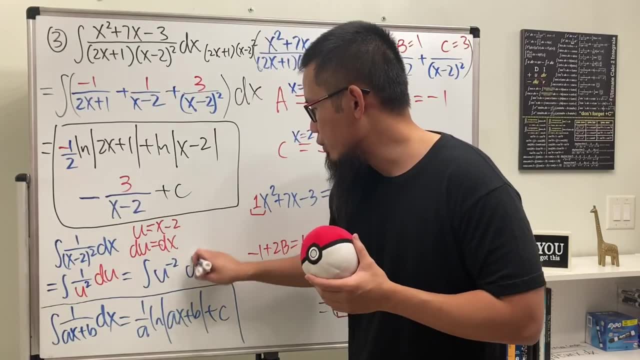 Square, the you right and then we're not looking at the bottom. right here, This right here. It's the same as integrating you to the negative 2 in the new world And again you see, we add 1 to the power. that will give us negative 1 for the new power. 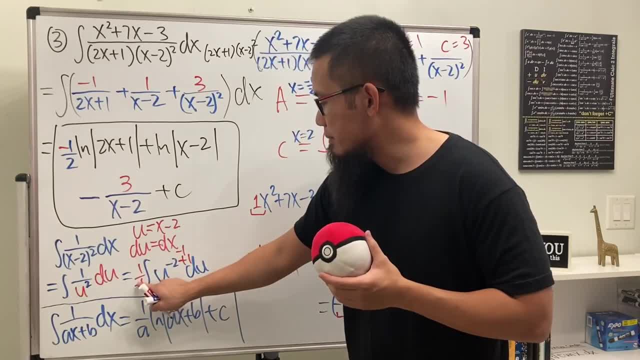 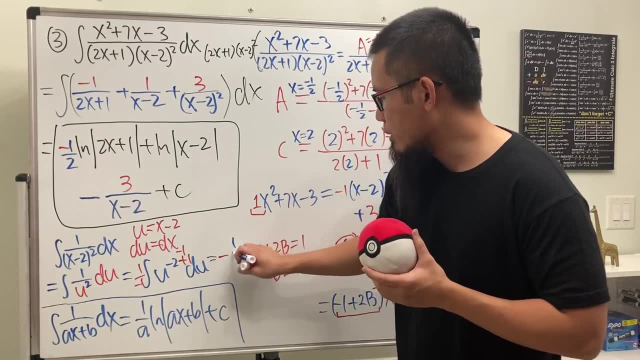 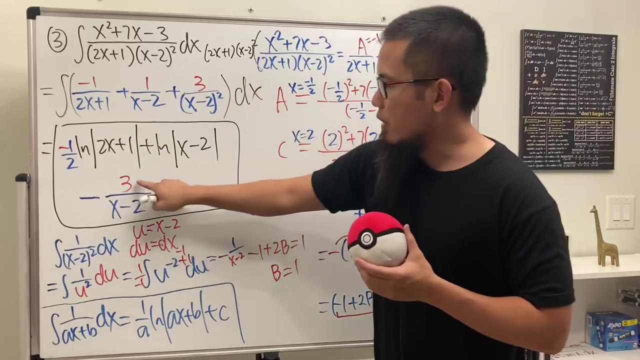 Divided by the new power. put it right here. That's why it becomes negative. And if you look at, we get a negative right here. And then u to the negative 1, which is 1 over u and you is X Minus 2, and that's why we have this part. And then this 3 is fun here. 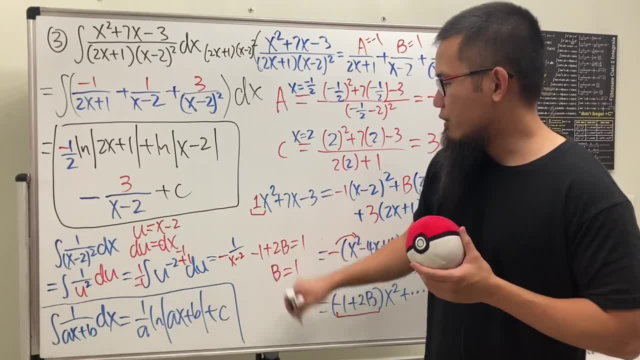 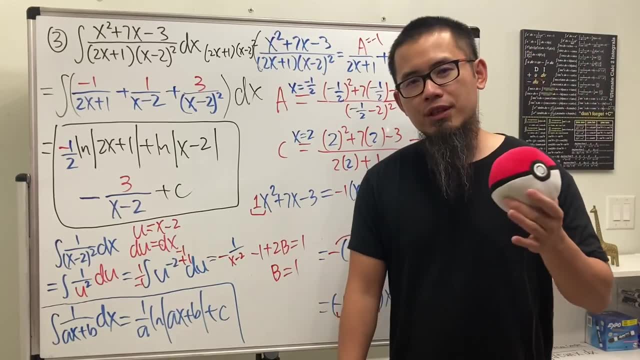 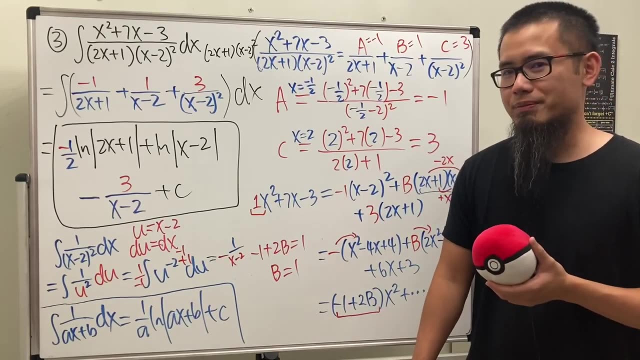 Alright, so just do the use up on your own whenever necessary, All right, So hopefully this video is for partial fractions are helpful. If you need help with calculus, you guys can subscribe to my channel. watch my other videos for integration. we're calculus to tutorials, as always.